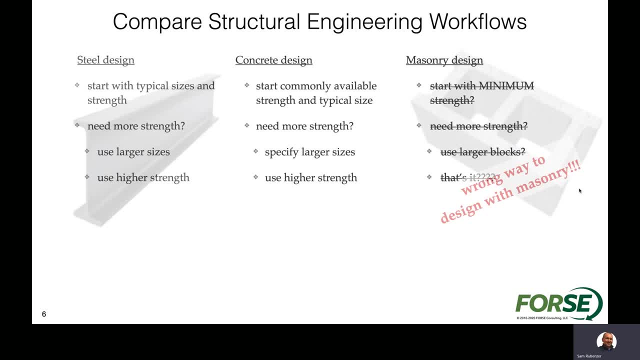 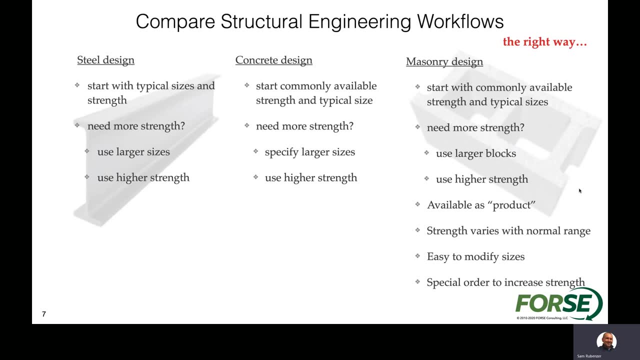 that we want to see masonry design being done. We really want it to be done on a similar perspective as what you look at for steel and concrete. You need more strength. use larger blocks First, maybe understanding what the actual strength is, before you can go to a larger block. 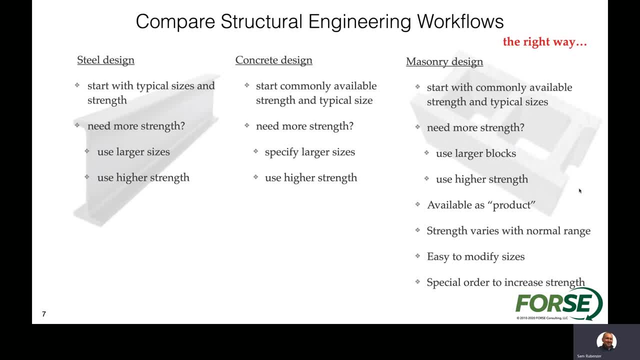 But then recognizing that you can also specify higher strength of masonry. You see, masonry is available as a product, which is kind of similar to steel. right, It's available as a product. There's producers that make the product. but what is certainly different from? 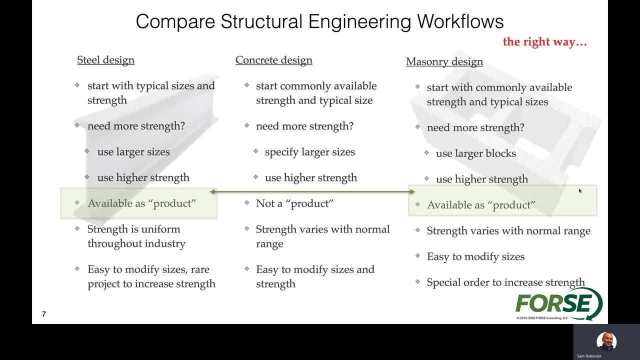 steel is masonry block strength is definitely different. See, I think the when you're using stronger- I mean stronger- masonry is going to tell you to improve the structure of the masonry. block strengths definitely vary within different areas of the country, different aggregates, different. 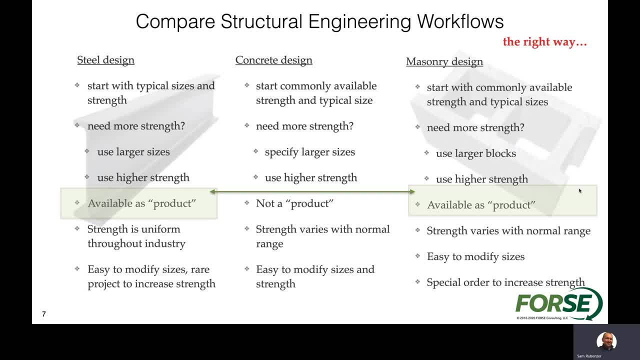 mixes from different manufacturers, So there's a variance with the actual structural masonry materials, somewhat more similar to concrete. It's pretty easy to modify sizes. You can certainly do a special order to increase strength, And so maybe that's where masonry is kind of similar to. 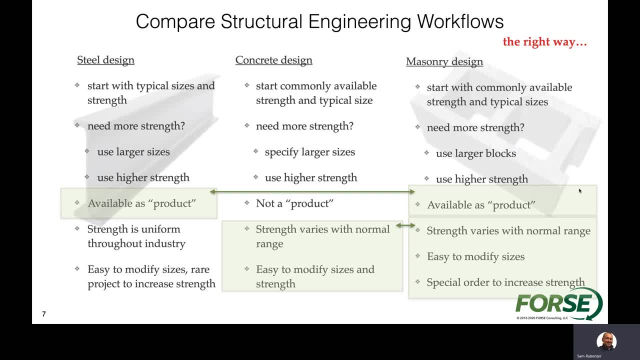 concrete design. If you need more strength, increasing the actual design strength- is something that we have available for masonry. So, really, what we want to do is elevate an engineer's understanding of masonry design so that we can bring it more in line with. 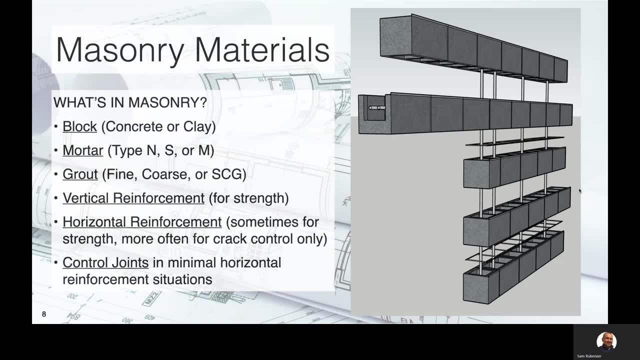 both steel and concrete design. So the focus for today: what's in masonry? What are the different masonry materials? We have blocks, which is obviously the key component, either concrete or clay units that we're going to use to comprise most of the wall. We have mortars that can come. 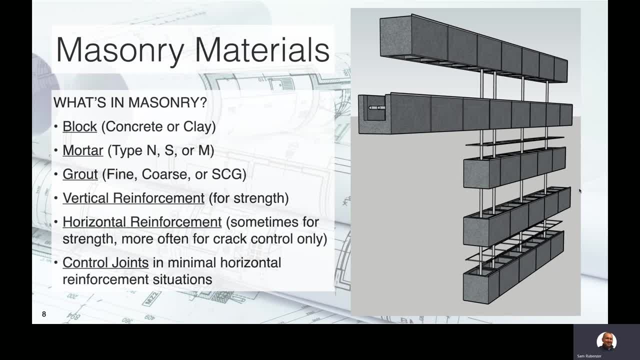 in type N. The lower stretch of the wall is the lower stretch of the wall. So we have mortars that can come in type N, The lower stretch of the wall is the lower stretch of the wall. So we have mortars that can come in type S or M with a higher strength mortar. We have grout. It comes in a couple different varieties as well. We have fine, coarse or self-consolidating grout. And then to reinforcement. we have vertical reinforcement. Typically most masonry elements span vertically, So that's vertical reinforcements mainly in their force strength. Horizontal reinforcement can sometimes be for strength, say for a horizontal spanning wall, maybe a masonry shear wall. We need some horizontal reinforcement. 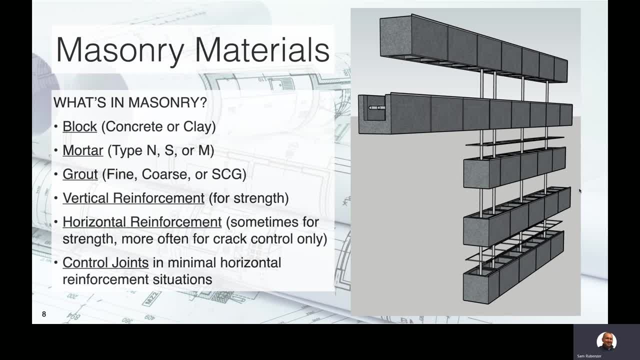 But most often their horizontal reinforcement in masonry wall is primarily there for crack control. Certainly in the Midwest and lower seismic areas crack control becomes very important for horizontal reinforcement And then, going with the horizontal reinforcement, another material that we have to understand is the materials that are used for creating control joints in our masonry walls. 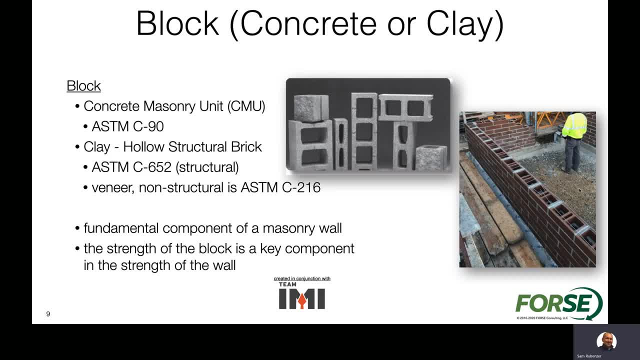 So first we'll start with block, Again, the concrete masonry unit governed by ASTM C90.. Which would be the primary masonry element. We have clay hollow structural brick, ASTM C652.. This is a lesser known material, but certainly something that's highly efficient and actually has incredible strength properties. 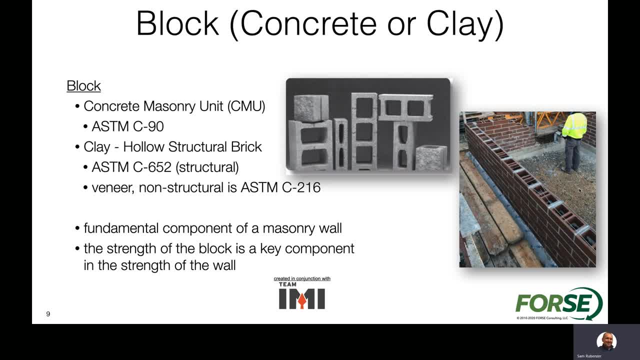 So both concrete and clay can be used as reinforced structural masonry units. Certainly, you also have clay veneers which would be non-structural. So I just want to make sure people don't get confused. You have clay veneers, non-structural, which would be governed by ASTM C216.. 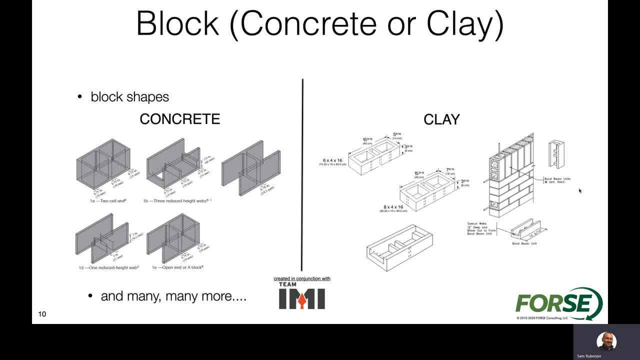 Block shapes something that we have to be familiar with as engineers. We have many different block shapes that are available. Certainly, different types of block shapes help us create different design elements within a wall. You have the standard kind of 2-cell unit that we would use predominantly within most masonry elements. 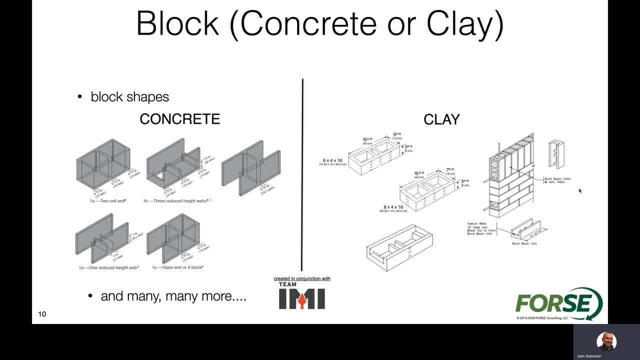 We have something similar for clay. We have two primary elements within walls, two primary cells for reinforcing, But then we also have bond beam units where we have some openings for the reinforcement. We have webs that we can knock out so that we can more easily. 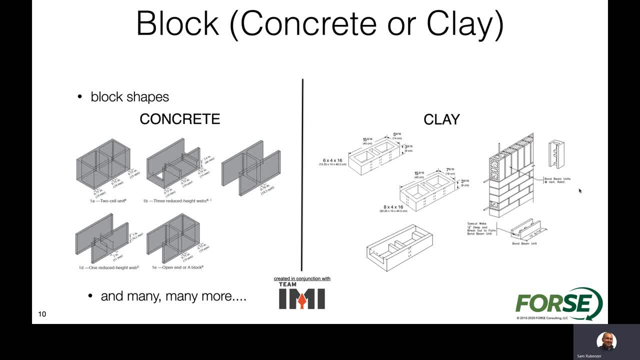 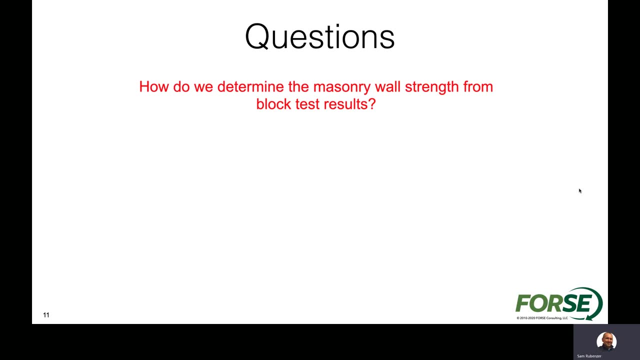 create horizontal reinforced elements within the wall, But then other specialty shapes, H-shapes or A-shaped blocks are also available, which was certainly important when we get into heavily reinforced masonry walls. How do we determine the masonry wall strength from block test results? There are really two different options: Prism testing or the 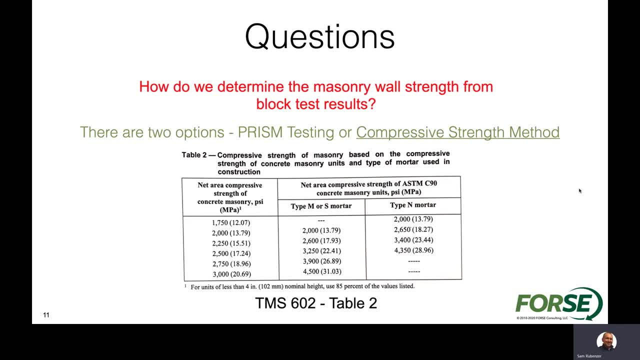 much more common compressive strength method. Compressive strength method is really just becoming familiar with a table from TMS, understanding what your actual block strengths are. Again, that's information that we can get from the actual block manufacturers And then the mortar that we specify. So once we have 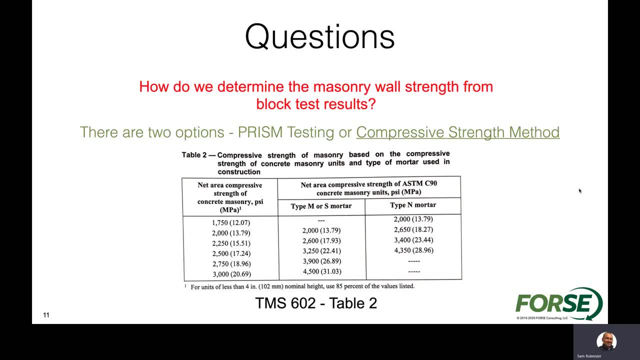 less than one block strength and the Broadway block strength. then we're able to generate the two different components. we really can determine what the overall net area compressive strength of the concrete masonry assembly would be. so we'll come back to this in a little bit and talk a. 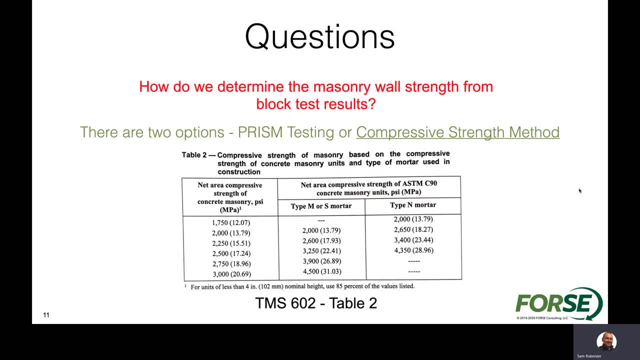 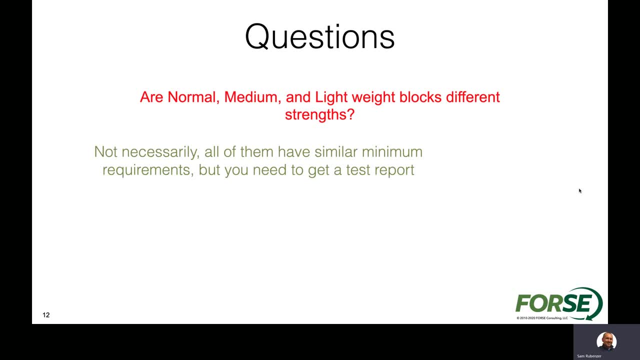 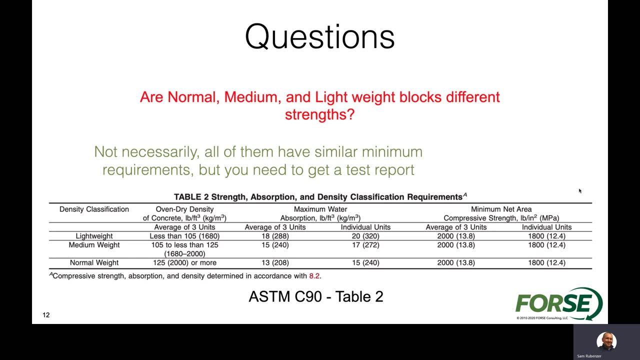 little bit more about what you can expect within different areas. another common question: are our normal, medium and lightweight blocks of different strength? and really they're not necessarily of different strengths? if you look at astm, c90, both or all lightweight, medium weight and normal weight blocks really do kind of rely on the same minimum strengths. so from there it really depends on again. 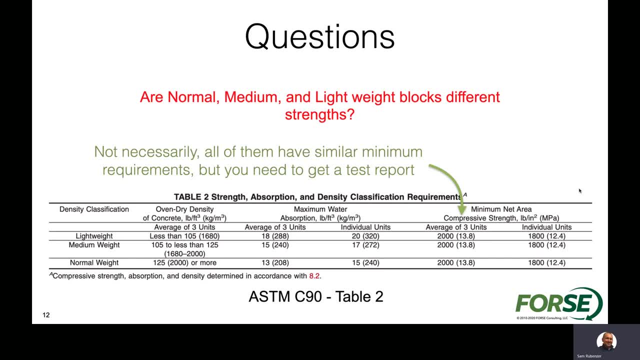 different block manufacturers and mixes and aggregates that are available, and so you certainly see some variants. i've seen lightweight blocks that are on the high end of strength for masonry design and normal weight blocks that can be all over the place, so you really have to have an. 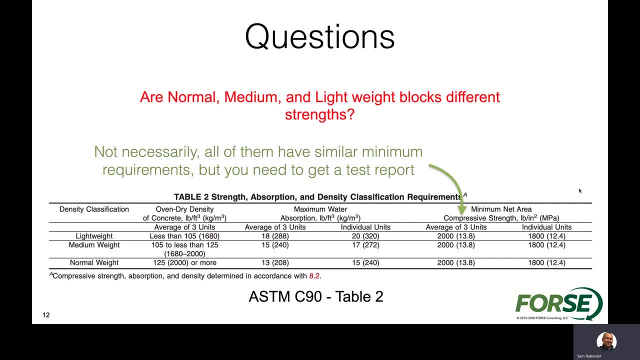 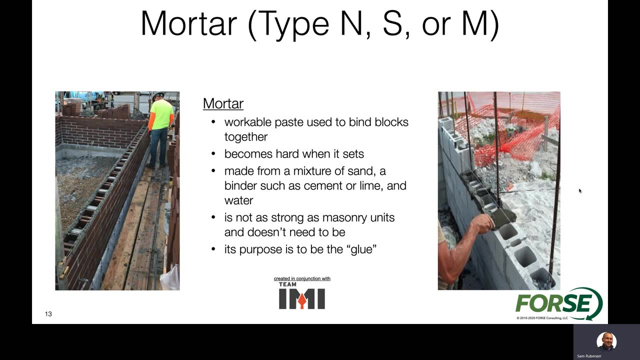 understanding for what the actual block manufacturer is making. it's not necessary necessarily the case that lightweight would be, say, less strong. next, within masonry, we have mortar, we have type n, s or m. again, mortar is really going to be the other primary element that you're going to see. so certainly architects care about what the color of 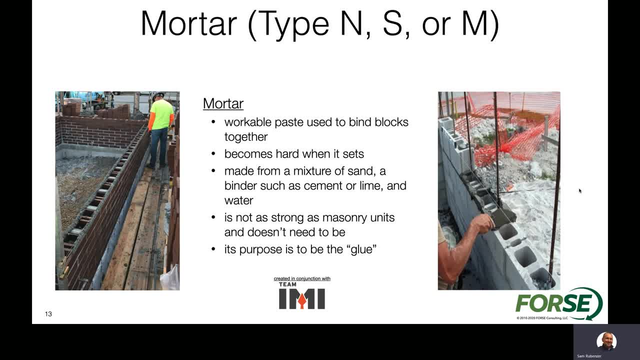 the mortar is perhaps to make sure that we have the right overall aesthetic for the wall, but from a structural perspective it's it's also very important to make sure that we have a workable paste that that binds the blocks together. it's going to be obviously a cementitious material. 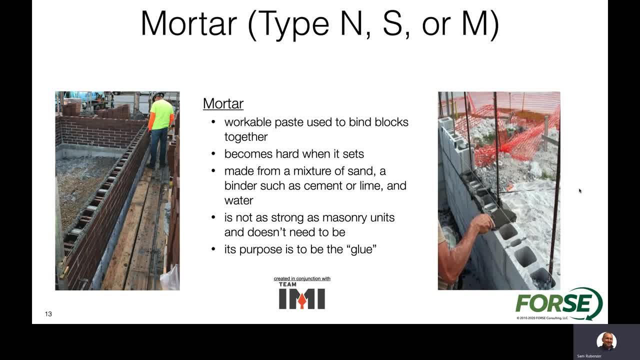 that becomes hard when it's used to build the wall, so that's something that we're going to look at when it sets. it's made of a mixture of sand and a binder element, such as cement or lime, and water- mortar- the one thing that i think is the most misunderstood part about mortar. 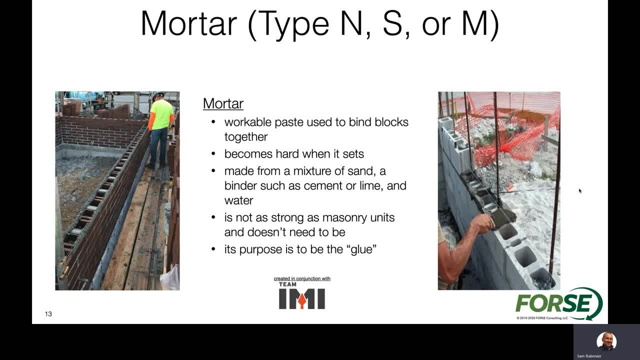 is the overall strength of the mortar and how it's tested. we really have to be careful that we understand mortar strength versus the assembly strength from the different types of mortar, because the strength of the mortar is really not a key component in the overall strength of the wall. 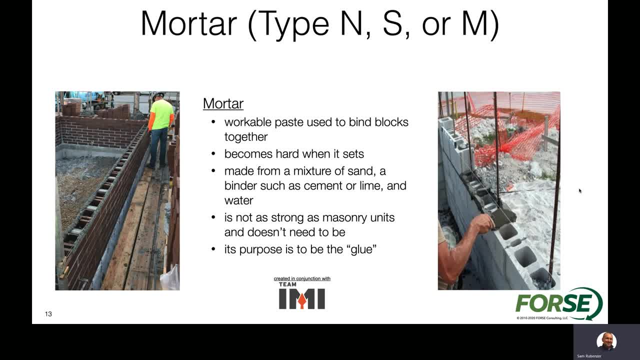 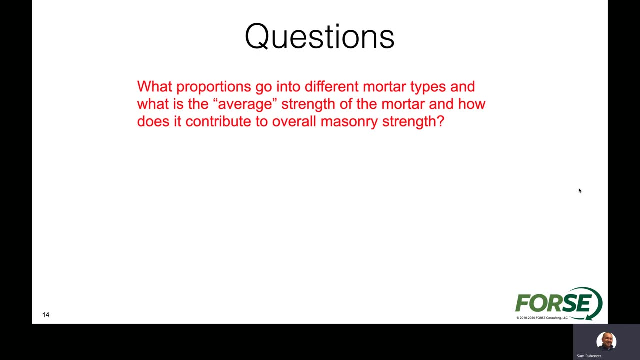 it does have a lot of different properties and it does change the strength of the wall. if you use, say, a really weak mortar, but it's, the wall is not as weak as the mortar, and we'll show that in a little bit here. what different proportions go into different mortar types? what is the average strength of? 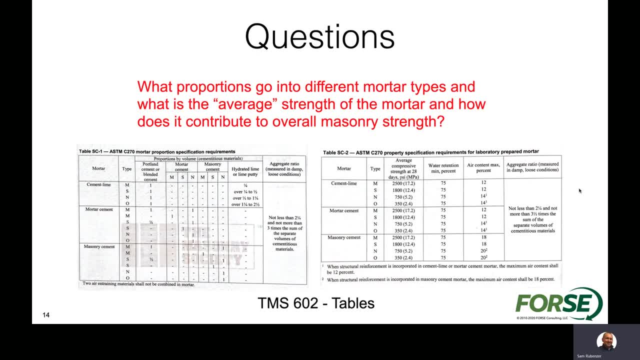 the mortar. both of those questions could be answered again within tms 602. you can see all the different types of ways that you can get different types of mortar, the ms's and n's also inside the structure on the core. it's the same thing you can see here. what I got here is 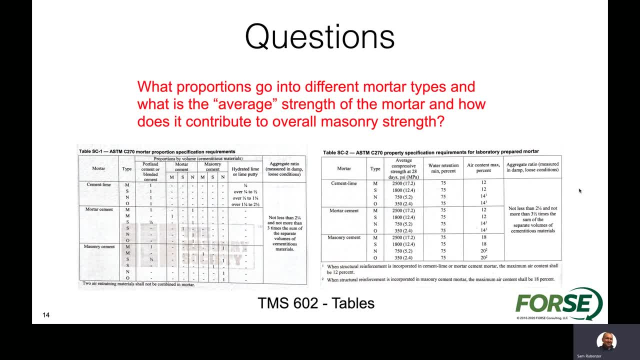 one type of mortar, a planer. we're not going to go into all those types of mortar, all of them, but you can see here just one type of mortar you can use for building a wall. so a planer is the type of mortar that you would use for building new walls. you can use for building 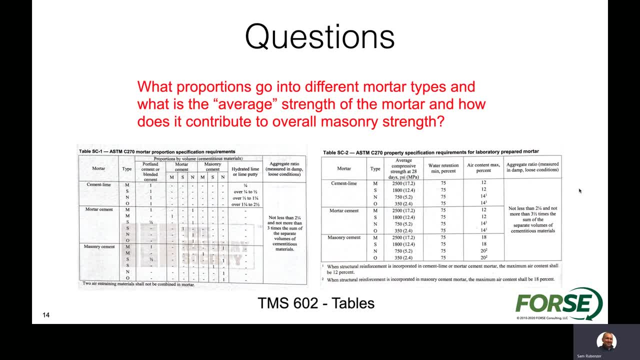 walls or if you were to do something that was not the same type of mortar. you want to have something that was really kind of on the the weaker end, maybe something that you would use for retrofitting. but you know, all those different type of mortars have a pretty much of a. 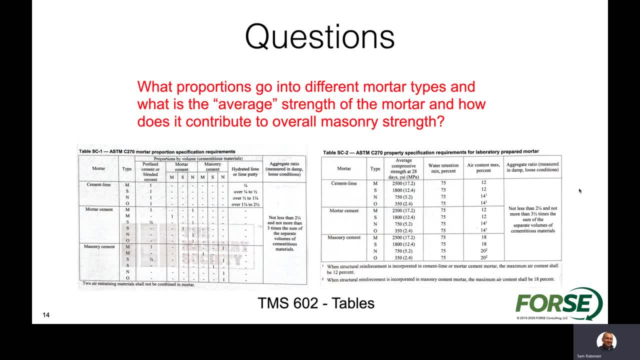 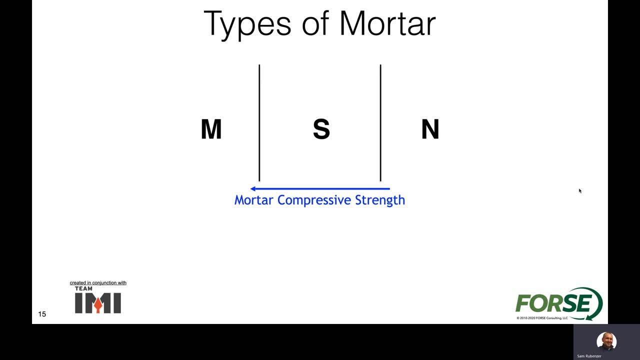 have some effect on the overall strength of the wall, but not nearly as much as what that column suggests. And so for the next slide here, what I really want to look at is again the three different predominant mortars that we see used within structural masonry. We have type M 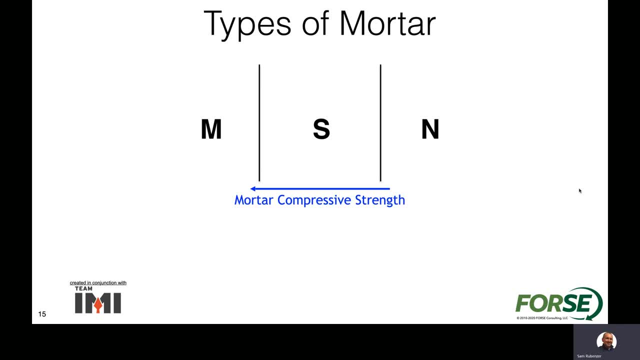 S and N. Really, the mortar compressive strength really does get a lot larger as you go from the right type N to type S to type M, which would be certainly the highest compressive strength for the actual individual mortar. But I would say that's a pretty small element or small component. 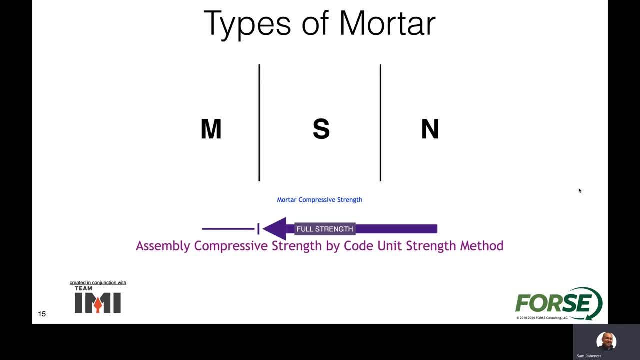 of the overall design because really it comes down to what the actual mortar, what it yields in the overall assembly. And you really can kind of see this by some of the testing that's done and what is given by the, the unit strength method, within the code When we go from type N. if we use that, we certainly have. 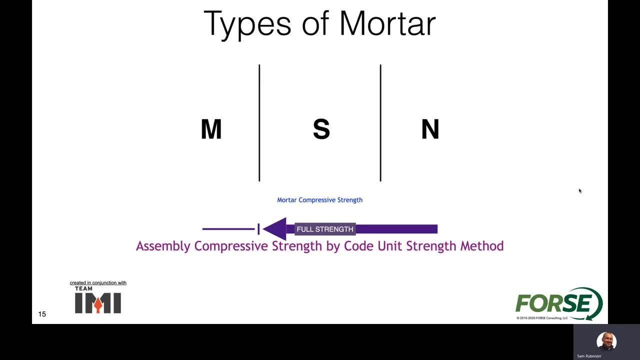 a less strong wall assembly, something on the order of 13 to 70 percent less strength, But using type S, which could be twice as strong as type N in terms of the mortar compressive strength. really, again, we gain a little bit but not a lot by going to that type S If we go all. 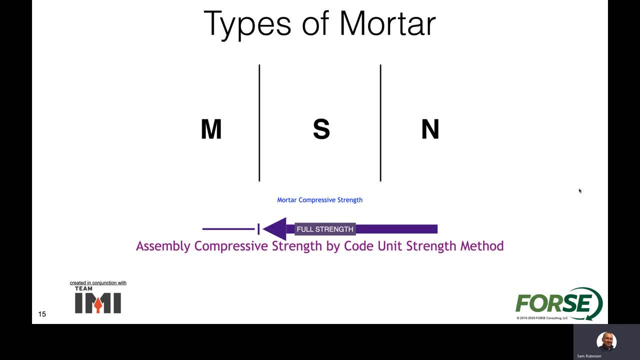 the way to type M, which again, sometimes you think, boy, that's going to be the the strongest mortar and that's going to be our best strength. you're looking at the unit, the code unit strength method. you can see that type M and S really do yield kind of a similar. 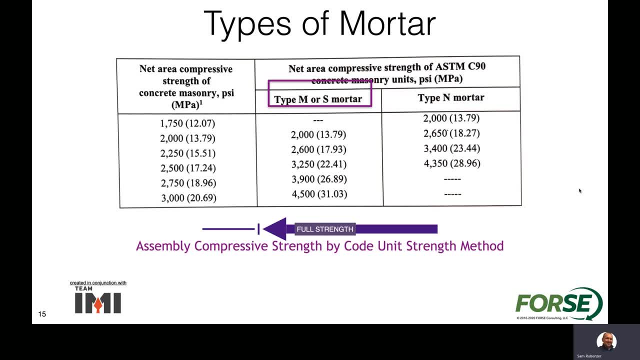 assembly strengths. In fact, if we go back to the table from TMS, you can see that they- the code just lumps them together- Type M or S, either one. if you use either one of those mortars, then we have the overall assembly strengths that you can see in the center column. So again, 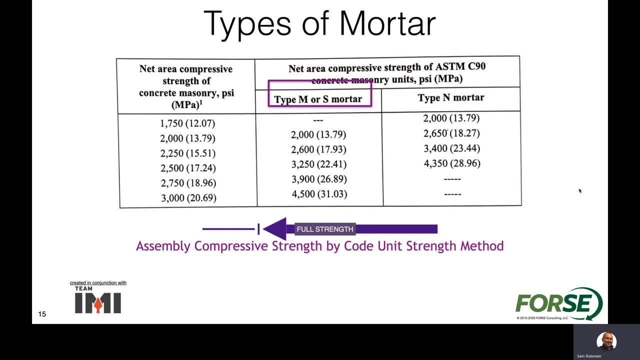 if there might be a little bit of lure to use the type m because of the higher strength of the mortar itself, but the overall assembly, there's really no benefit to going all the way to type m. type s is really going to get you as far as you need to go in terms of the overall assembly strength. so really, really, 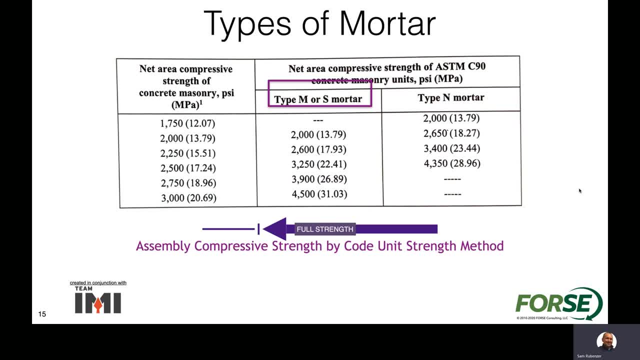 important to realize that there's, you know, and if you're thinking about kind of what i'm saying here, you can see that there's really not a really good reason to use type m, um. for most, uh, mainstream designs, type s is probably going to be um. the more that you want to use really f, prime m is. 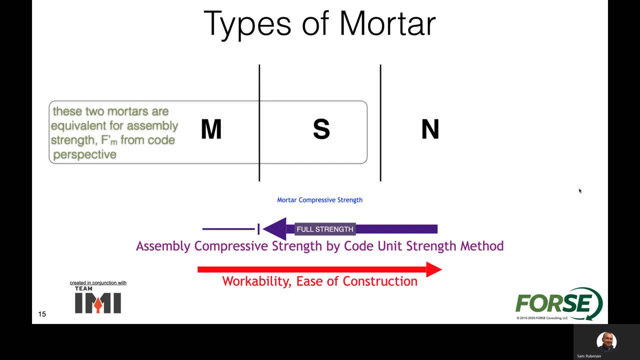 going to be the same from the code perspective, you know. and the reason why not to use type m? because it's it's not that easy to work with. it's it's the workability issue for type m is is somewhat low, so using something that's a little bit more workable- masons like to use type s a lot. 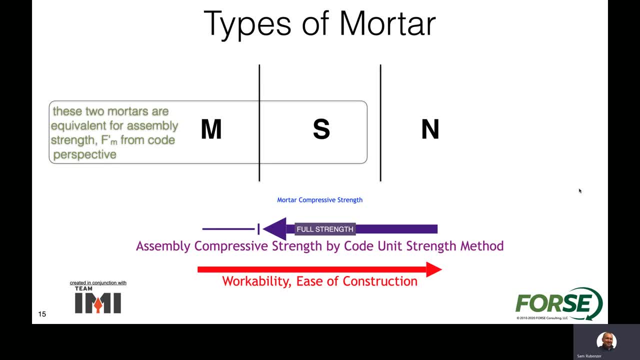 more um. so really we want to take that into account as we specify these mortars as well. so i think really good way to remember it is: use type s for structural. it's really going to get you most of the properties that you're looking for and be something that masons are going to be. 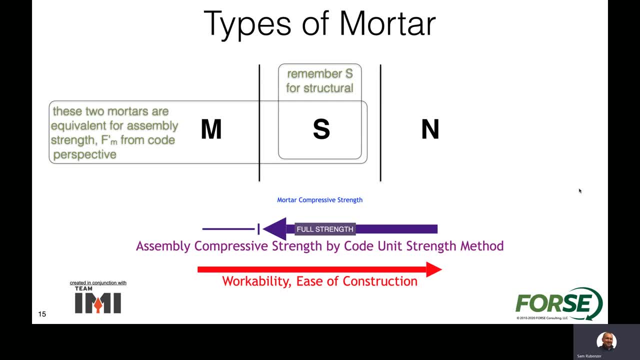 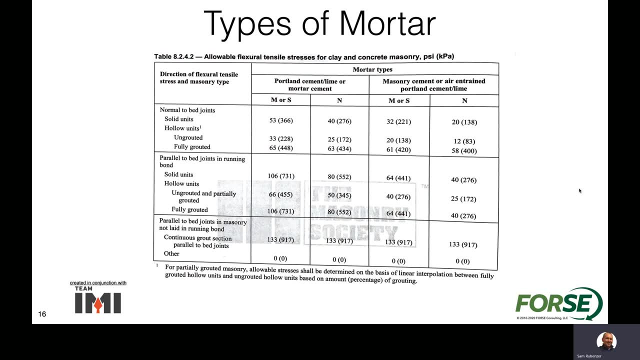 used to using and like using as well. the last thing that i want to mention on mortars here is just looking at the overall tensile stresses for the different types of mortar. again, mortar cement, masonry cement have different types of properties, so they have different types of. 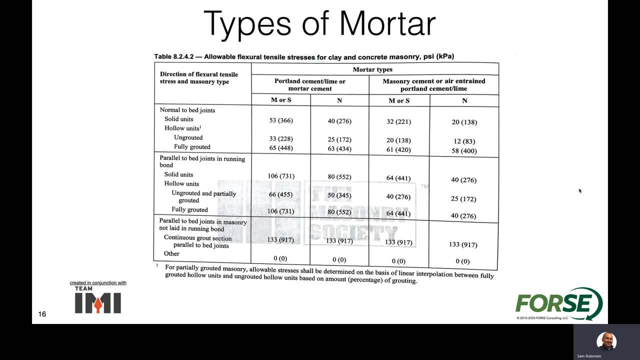 mortars. so we want to make sure that the type s that we have especially are not more than 40% more tolerant. where is the lower tensile strength? where is this going to be important? anytime that you get into an unreinforced masonry wall, we can still design unreinforced masonry. 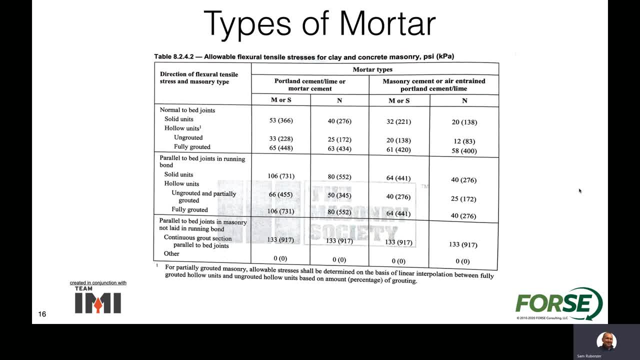 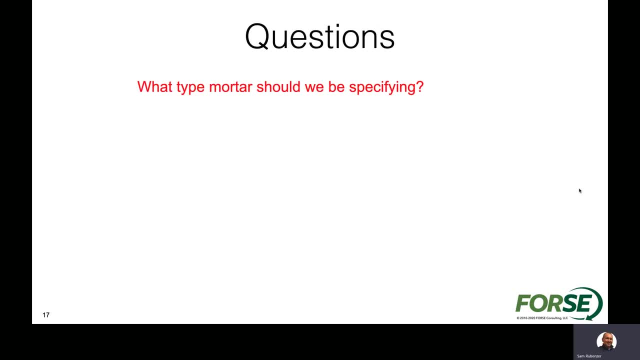 certainly for stuff like partition walls if you want to get the most out of your unreinforced masonry design. looking at mortar cement is certainly be a good idea, as you can see some of the tensile values here higher for those types of mortars. the three different ones: you have type m, which is a high strength but more costly, reduced workability. 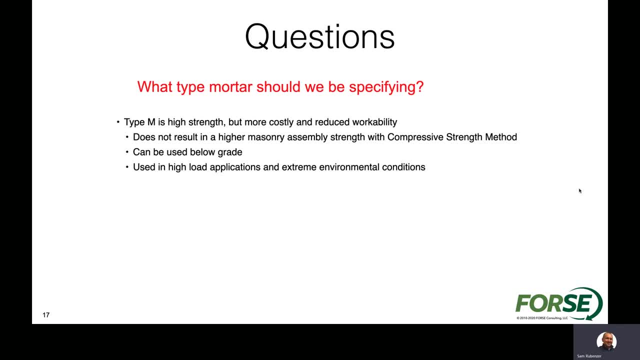 really doesn't result in a higher compressive strength. it can be used below grade. it's really kind of reserved for those very high load applications or extreme environmental conditions. again, we recommend using type s as much as possible for structural walls, can be used in hot, all seismic design areas and it also can be used above and below grade. so really type s can be. 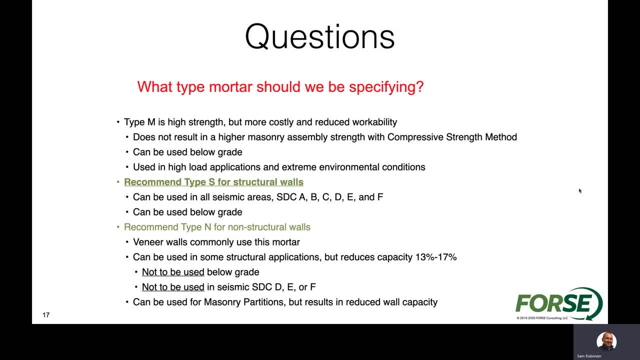 kind of the main mortar that we would like to see for structural designs. you certainly can use type n for structural, but it's more common for the non-structural elements, for veneer walls or lightly loaded structural elements like partition walls which would have a reduced wall capacity. the other 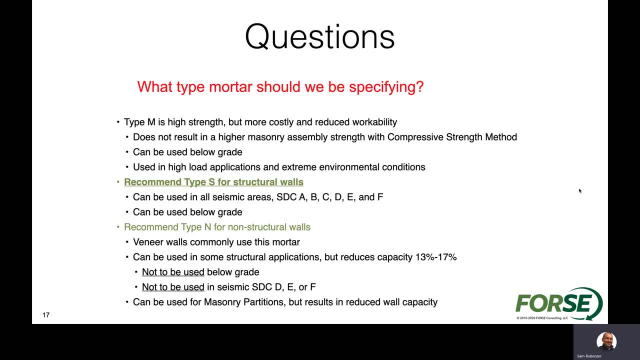 thing about type n is, if you did use it in the past, recognize that if you go into seismic design categories d, e and f, you wouldn't be able to use type n, and also you shouldn't be using type n below grade. so certainly some limitations there that we want to be cautious of. 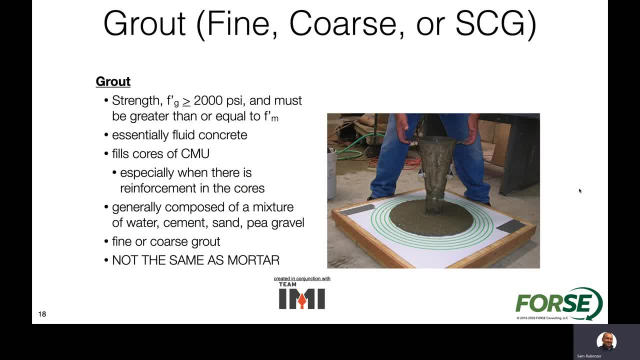 grout. the thing i say about grout is it's certainly much different than mortar. it's not same as mortar. it's got a very different purpose. mortar really meant to be the glue that holds the units together and, as you're constructing it, grout has very different purpose. it really needs to be. 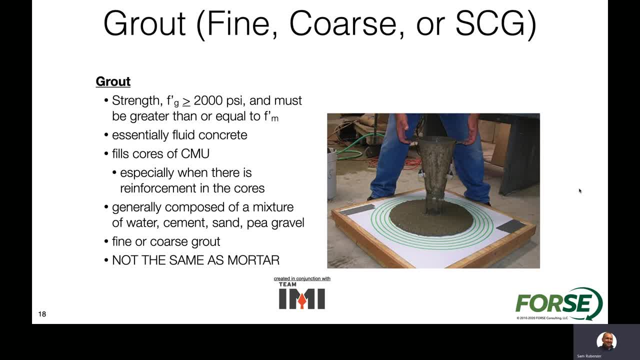 the fill that fills up your masonry wall. it needs to fit in within the cells of masonry. it needs to fit in within the cells of masonry so that it can flow around the reinforcement- horizontal reinforcement, vertical reinforcement- and then not leave any void. so it's really going to be. 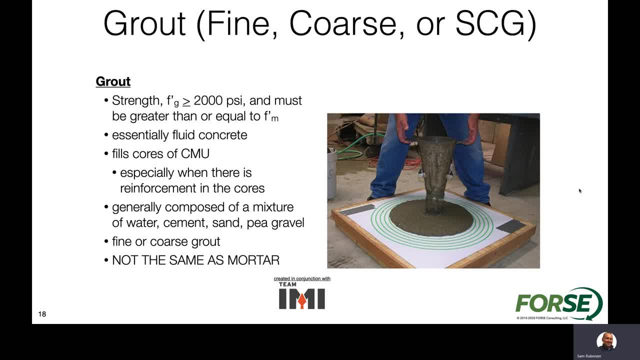 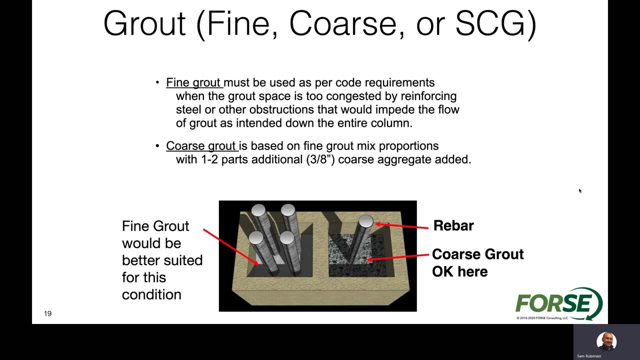 a fluid concrete material filling the cores of the cmu is again going to be composed of water, cement sand and some sort of a pea gravel. there's a finer, coarse grout that you can be using, and really finding coarse grout really comes down to what are the spaces that you have within the actual 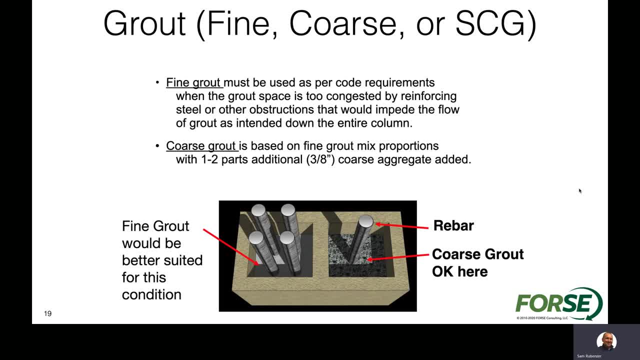 masonry cell do we have a lot of clearance so that coarse grout can fit in around. for most designs where you'd have a single bar, as you can see at the bottom, the coarse grout is going to be just fine and that's going to be. 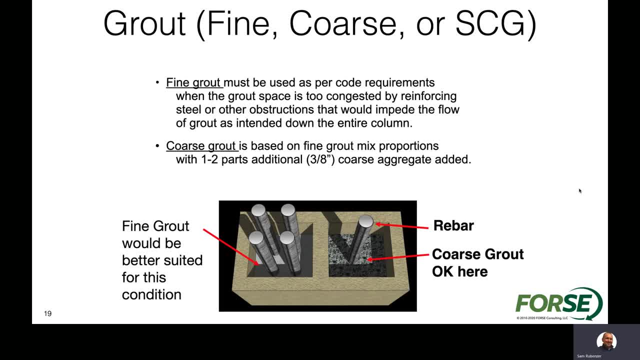 the predominant design for mainstream. there's going to be times where you get into, say, more of a column element or something that's going to have more reinforcement, kind of packed in a cell- certainly not something that's common within mainstream, yet isolated elements maybe that have this. but that's where you use that fine grout. you have small clearances between face shells and rebar. 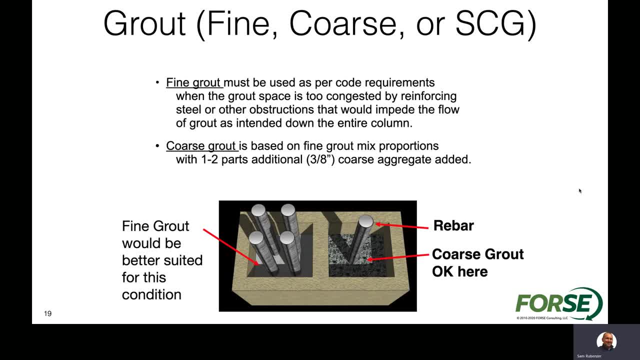 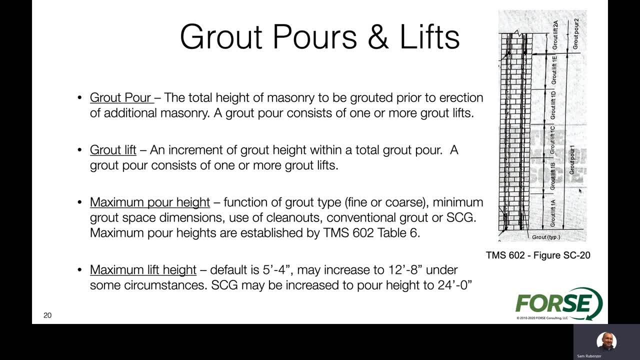 and you really have to be careful in what you use there. the other thing about grout that engineers tend to get involved with is grout pores and lifts. there's a really nice guide within tms 602 that kind of shows you the difference between pores and lifts and really this is a means and methods. 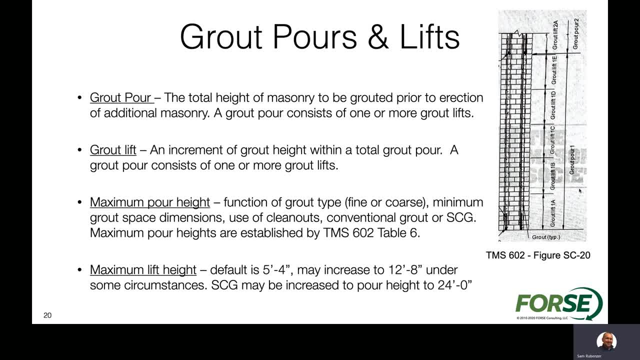 element. sometimes i see engineers specifying this within general notes. it's not something that's required for them to specify within general notes. you can certainly maybe provide some guidance, and that can be done right away, and there are a number of different ways to do that, i think. 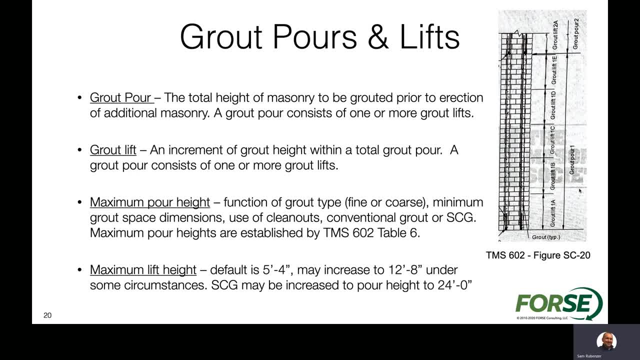 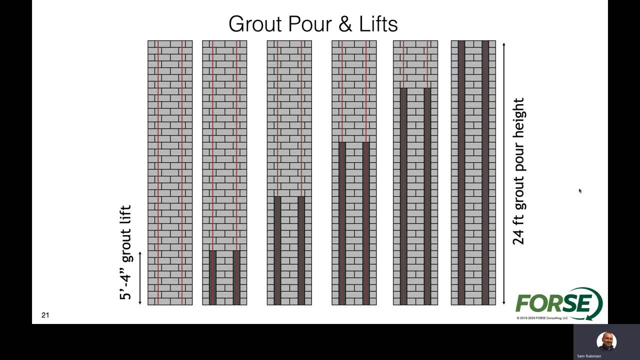 that's really important and that's why i think the the grouting options i think is really important because there are several different ways to achieve the grouting for a mainstream wall, depending on different construction techniques. you can see, you can use a five foot four grout lift. 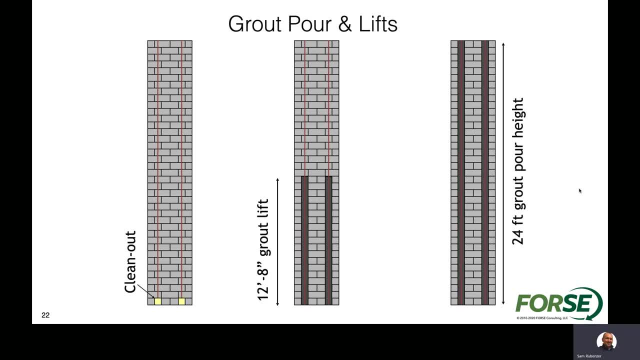 and so for 24 foot high grout pour you'd have several different stages that you'd have to build up the grout in that, in that wall, 12 foot eight grout lift and then all the way up to 24.. You can even use something like self. 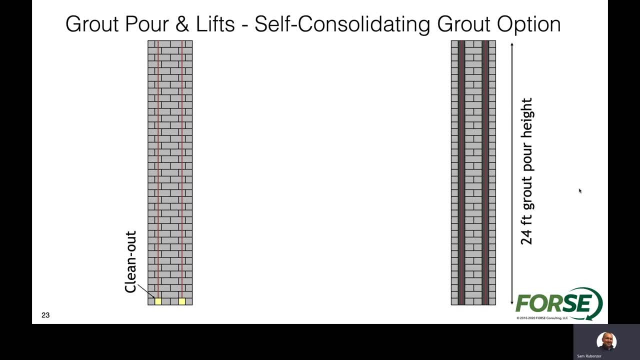 consolidating grout. So again, you can see the different options that are there. Contractors within different areas of the country, or just different means and methods, maybe prefer one of these over the other And I would say, as engineers, we just need to be familiar with. 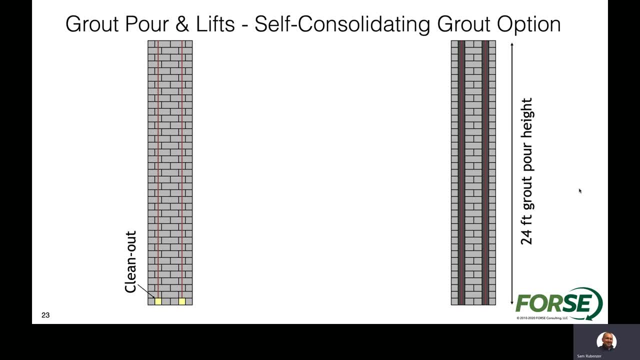 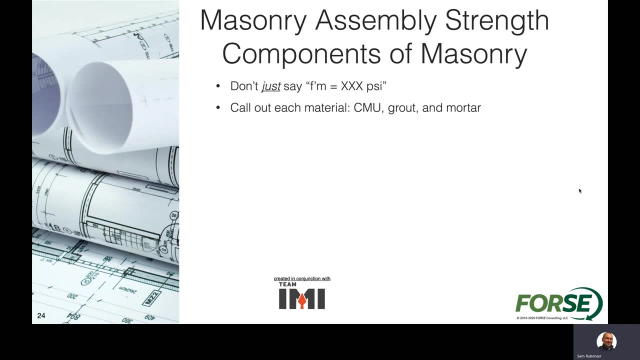 the different provisions and make sure that if we have a contractor that would use one of these different methods, that we understand the method as they've been clearly defined within TMS When we do specify masonry- one of the things that I like to see when I review. 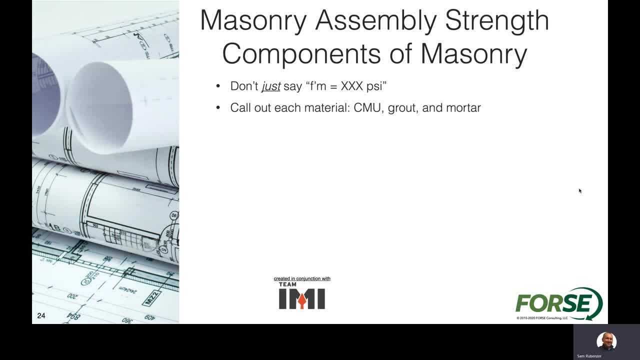 masonry general notes is. I like to see information about all the different elements of masonry. I don't like to see when engineers just call out a strength of masonry because, as you could see in the previous slides, there's different ways that you could achieve. 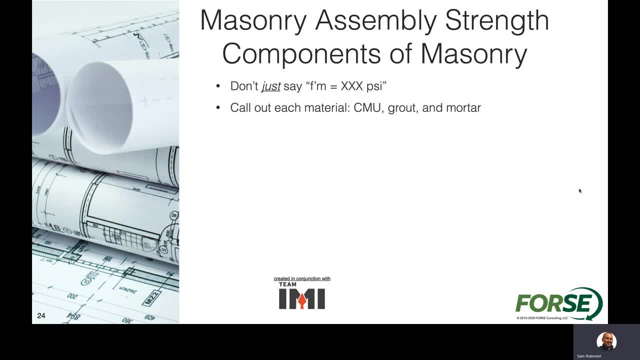 masonry. So I like to see when engineers just call out a strength of masonry because, as you could see in the previous slides, there's different ways that you could achieve a certain assembly strength. higher strength units and lower strength mortar could achieve the same design strength as a lower strength units and higher strength mortar, But maybe 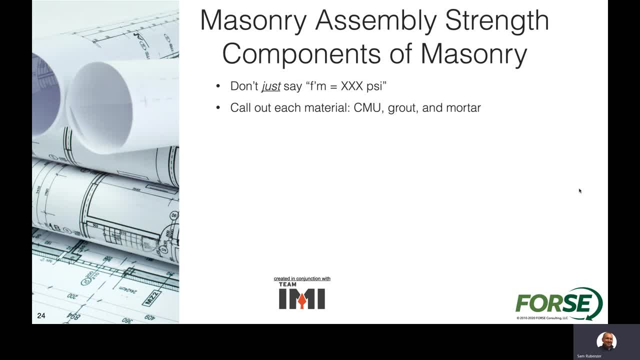 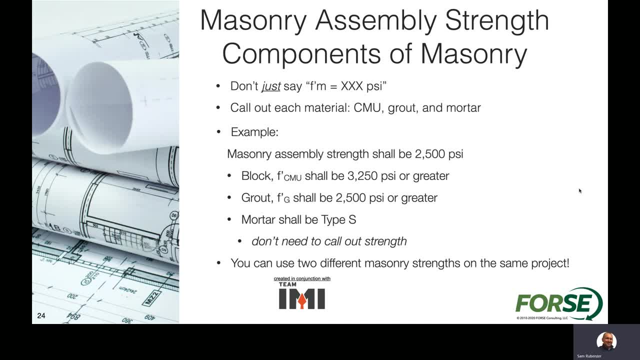 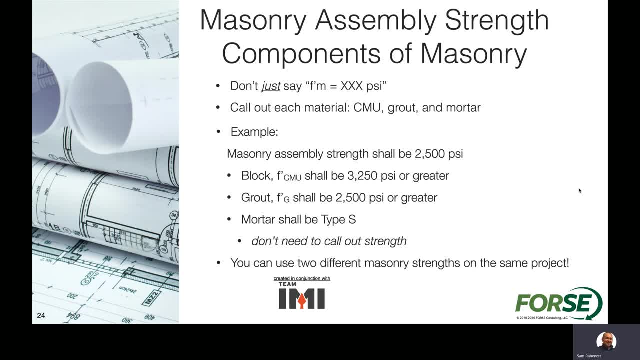 m of 2500 PSI. To do that, you need to have a block of at least 3250.. Very specific. We know exactly what we need now for a block. We have a certain mortar type, because I want to use type S. 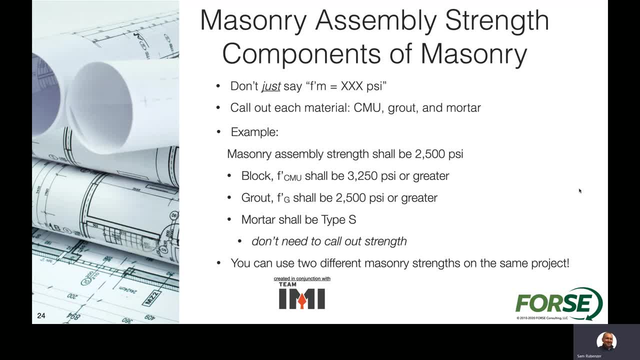 below and above grade. So we're going to call it mortar as type S, And then, based on that information, we know that a grout also would need to be 2500 PSI, because it needs to be at least as strong as the F prime, m or greater. The other thing is, you know, and I don't see this- 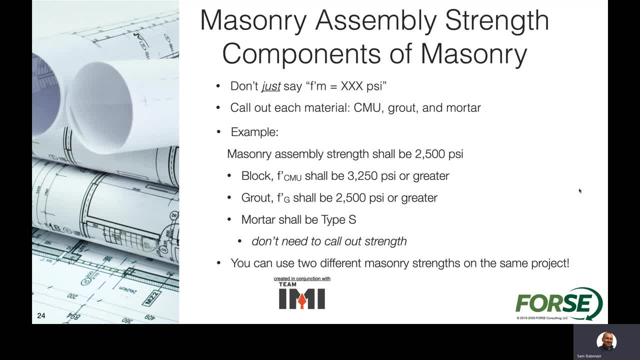 too often, but from time to time I'll see engineers that will specify two different masonry strengths. Maybe we have a large school that can use the standard F, prime m, Maybe that's 2500 for a particular area, But maybe we have a storm shelter that's going to be a very heavily 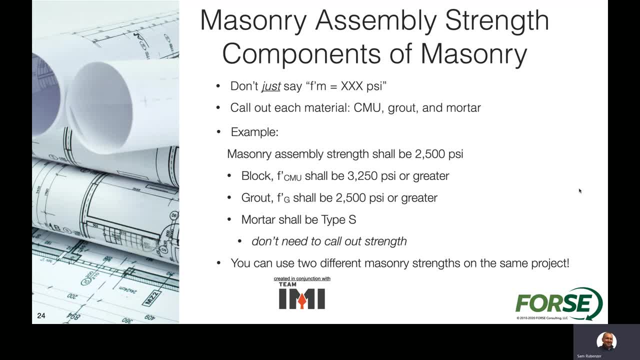 loaded storm shelter And we're going to have a storm shelter that's going to be a very heavily reinforced part of the actual design where we maybe want to use an F prime m of 4000. Something we're going to have to have a lot higher demand on that masonry within that same project. So use 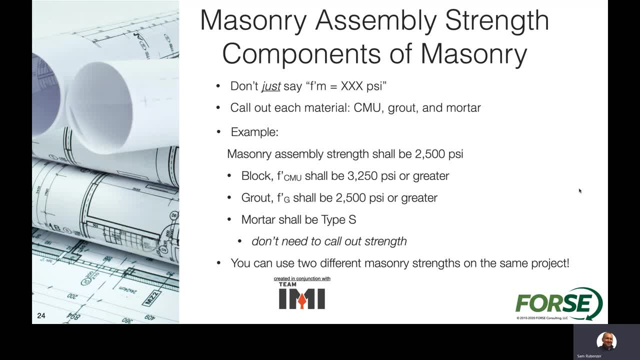 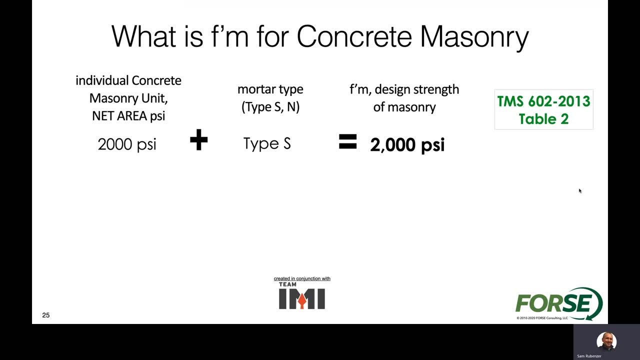 two different masonry strengths, Specify them on the project drawings. Call the different parts and components that would make up the two different masonry design strengths on your project And the contractors can follow those as they go into the build. Again, just kind of a. 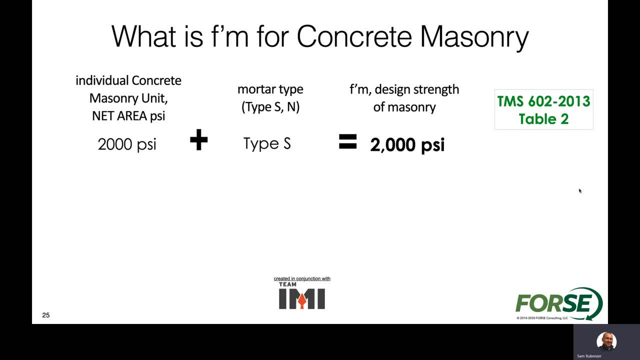 quick overview of what the F prime m is. Again, it's just based on your unit strength type of mortar Within the TMS 602, it gives us the minimum right strength of block of 2000 using type S. for structural type S mortar We're going to have a minimum design strength of 2000.. So 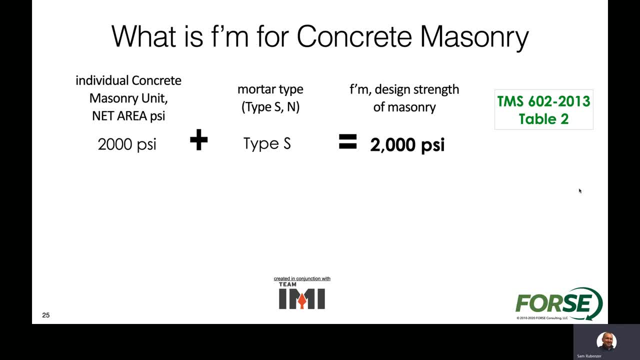 anybody that might be using something less than that. just recognize that the code since 2013 has been stating the minimum design strength for masonry with type S mortar. it's going to be at 2000.. So we definitely need to be at 2000 or above. And what I would say for 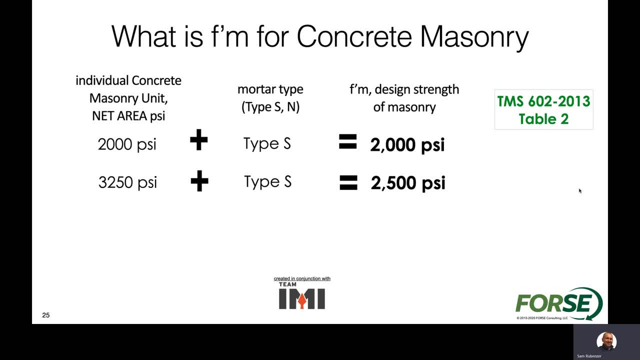 most of the designs in our country we can use actually a higher strength block, type S mortar. I'd say the most typical designs are going to be around that 2500 psi. That's going to be the most predominant design strength across the country. Certainly different companies offer blocks that. 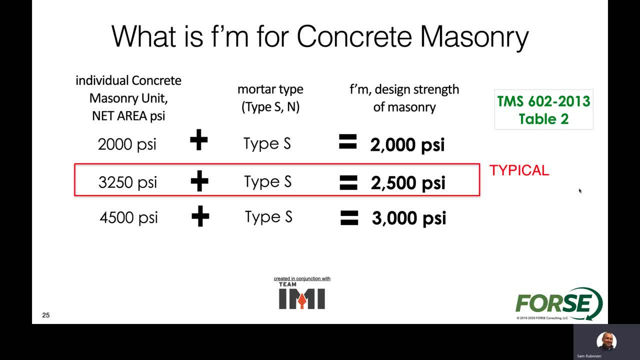 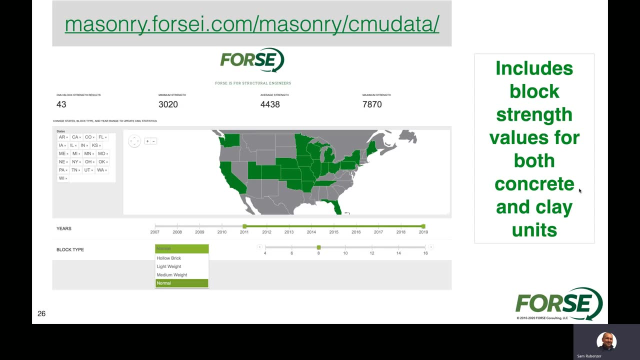 are even stronger: 4500, with type S giving us that 3000 psi. How do I know this? How can I make a statement that most of the designs are at 2500? Really, again, remember that 3250 of psi. what we've done? 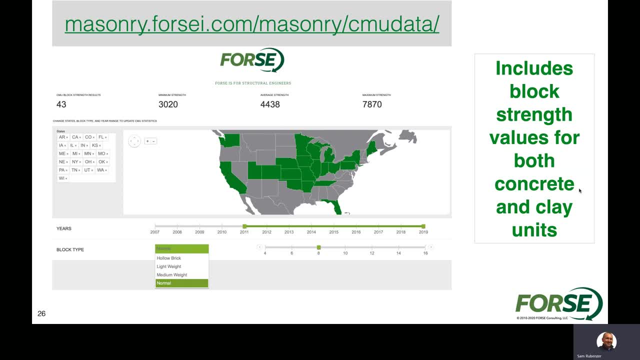 is, we've did some research and determining what some different block strengths are from the major block manufacturers and in many different states of the country. And again, if you look at the this map, we're just providing all those different block strengths, 43 different. 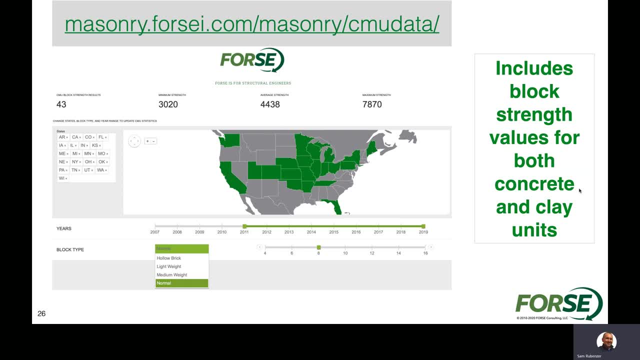 block test results. here for normal weight block. you can see the average strength. average strength is going to be in the middle of the screen, average strength being at 44- 38. so that's a lot higher than that- 32- 50. we can see that the 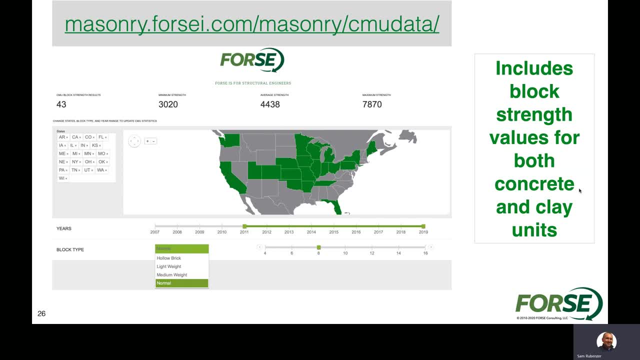 average all across the country is going to be a fair amount higher than that. actually, the minimum strength for all the different block manufacturers is 30- 20 again. it's not to say that we can't find a block manufacturer somewhere in the country that makes less than that. we still have to do. our research. but we should be confident in designing to an f prime m of 2500 throughout the country. we can run into those situations again if you get into the higher strength masonry. i mentioned 4000 psi before. we are going to have to make sure that we make special note. 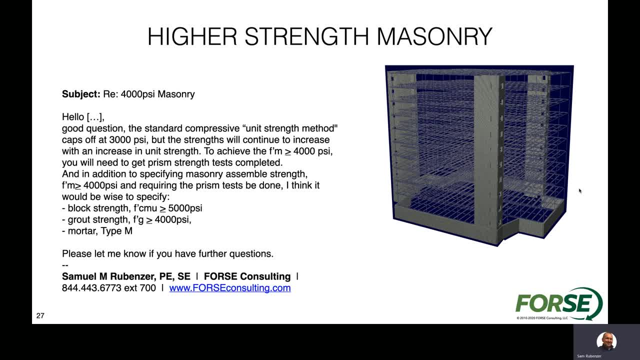 of what the actual block strength is: a higher that's going to be higher than 4000. maybe block strength for 4000 psi design. maybe we want block strengths to be around 5000. maybe in that situation it's a higher load demand situation. maybe that's when we use that type. 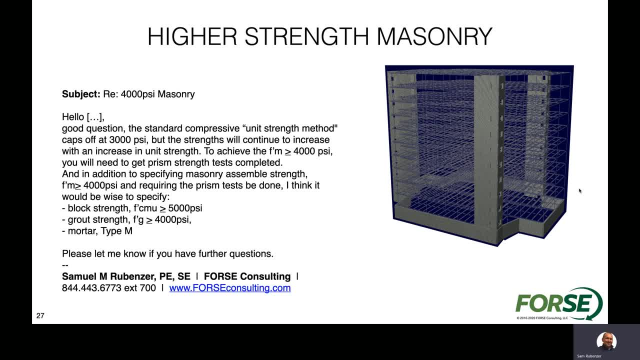 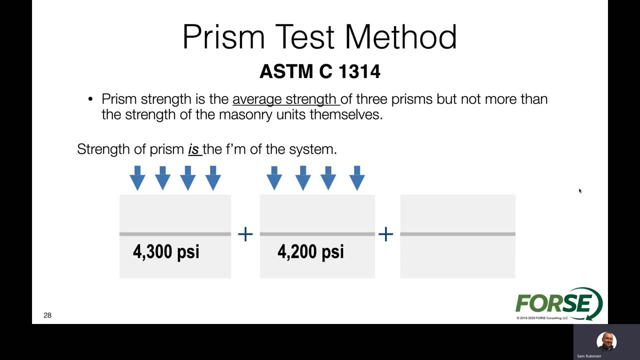 m order. so again, specify all those different elements. but then really, once we do that, we have to rely on a different method for the strength of masonry. we're going to have to rely on that prism test method. well, we really build three different prisms with the materials. 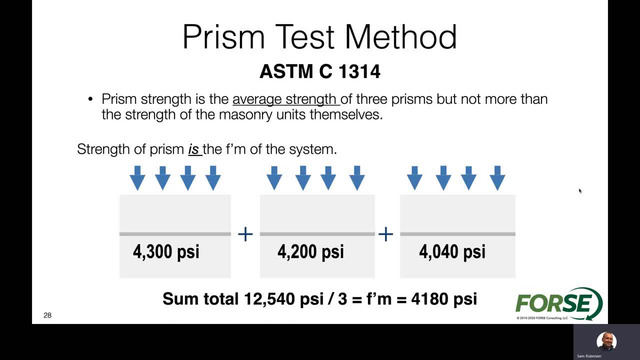 that we anticipate using for that design. we do some load tests for those different prisms. we average them out to elements, all test with an average that's going to be above the f prime m that we're specifying. so pretty easy to get there, pretty easy to understand how we can do some of this testing. it's pretty. 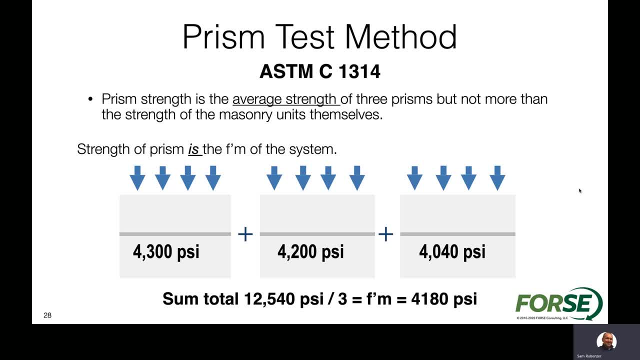 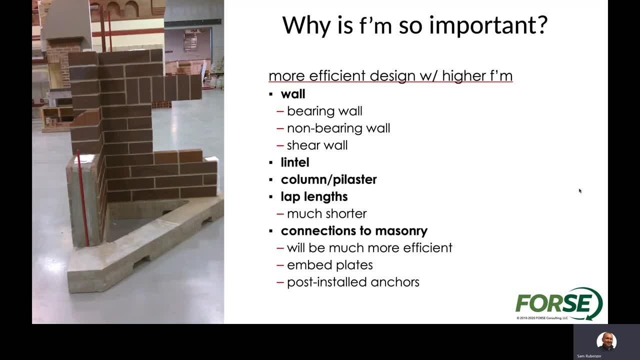 simple. it's not that costly to do this, so don't be afraid of recommending some testing for a higher strength design area. and again, why is f prime m so important? it's certainly going to be something that leads to a more efficient design. f prime m is important when we have an element that we have. 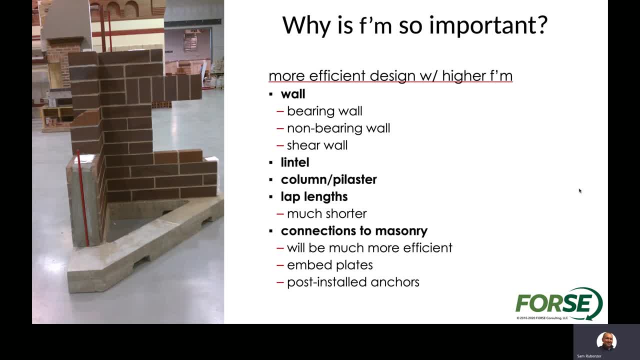 higher load demand. so we're going to have a higher load demand, so we're going to have a higher load demands on. so walls are going to be your predominant element. bearing walls, non-bearing wall, shoe walls- they're all going to be a little bit more efficient with f prime m. you know tall. 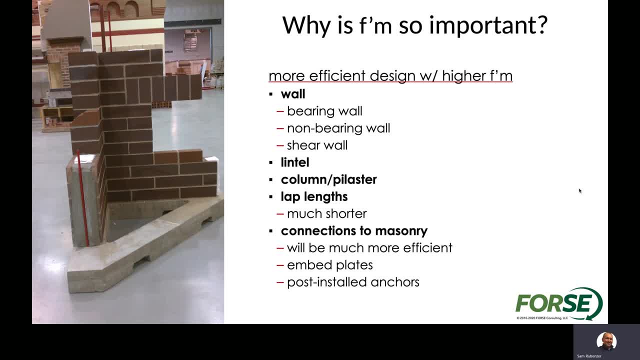 slender walls. oftentimes a lot of people tell me: well, those don't really change, sam, when you know, i increase my f prime m. now that's fair enough. but the lintels within that tall wall certainly do change. lap lengths get a lot shorter within that tall wall with a lot of reinforcement. that's going. 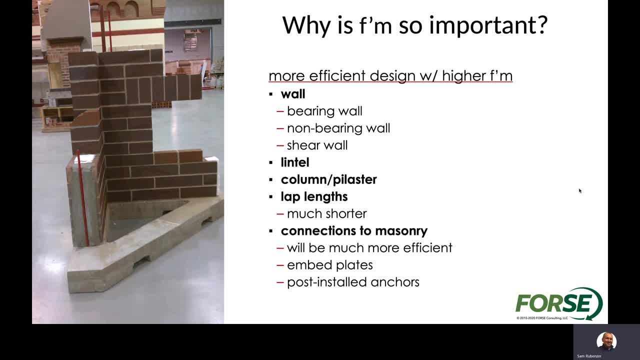 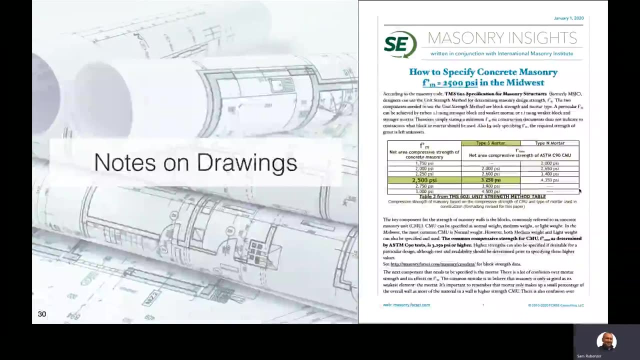 to get a lot more efficient and then all the connections to those tall masonry walls are going to change a lot more efficient when we recognize the right f prime m. so there's plenty of incentive to understanding what the f prime m is. recognize that it's 2500 or higher. actually created a white paper. 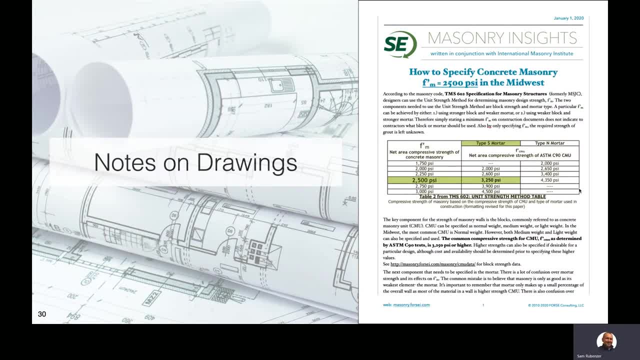 for the midwest, recommending 2500 for the f prime m. this this paper is certainly available. you can certainly request that from any imi representative or from myself as well. so f prime m is certainly important and we really need to understand what it is to get a good and efficient masonry design. 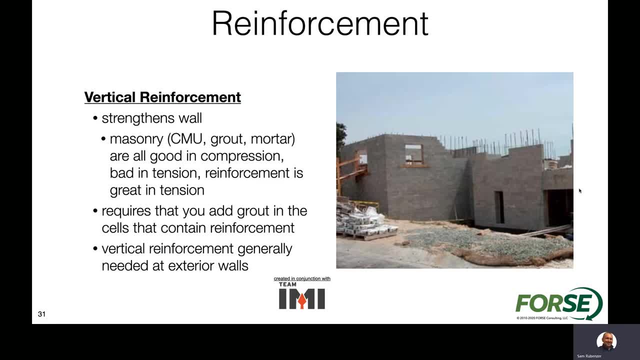 last couple elements here for our masonry wall materials: vertical reinforcement- again it's going to be what's going to be. strengthening the walls- can give you a lot more capacity in your wall. certainly, if you add reinforcement, you need to make sure that you add grout in those cells. that's a. that's a pretty straightforward application. 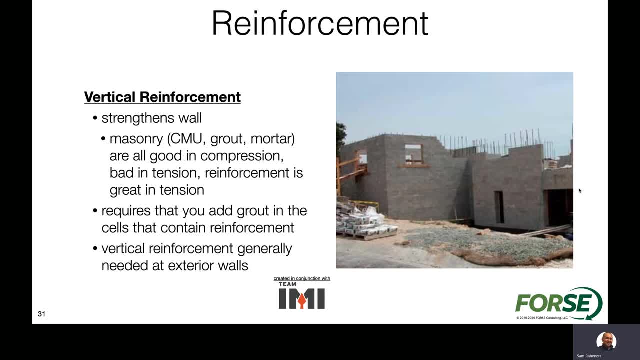 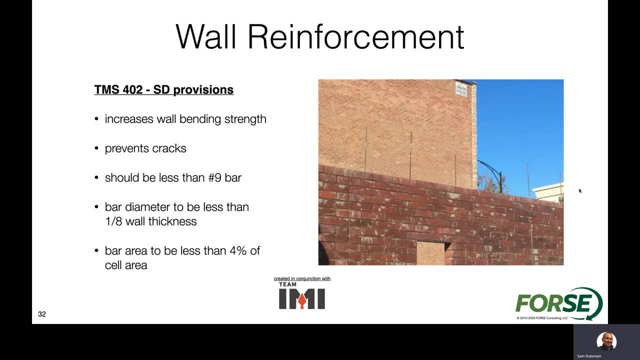 and typically vertical reinforcement is going to be used in exterior walls. you know, within the code there's also some pretty good indications for what amount and size of reinforcement you want to use. within the tms 402 strength design provisions it recommends that bars be number nines and less. again, you think about mainstream walls and you think about how. 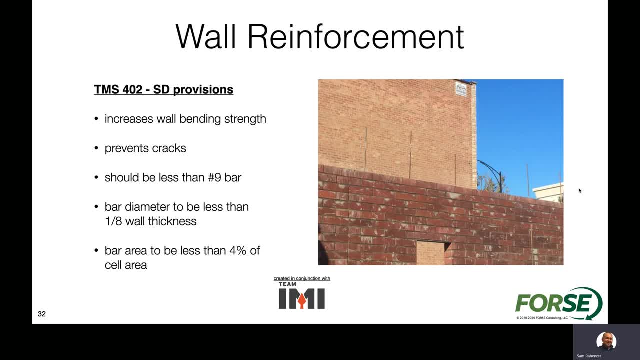 we have these confined spaces. putting a number, nine bar, is going to be a challenge in itself, so recognizing that we don't want to use something anything larger than that. a bar diameter is to be less than uh eighth of the wall thickness: again small, smaller, thinner walls- uh, even less. 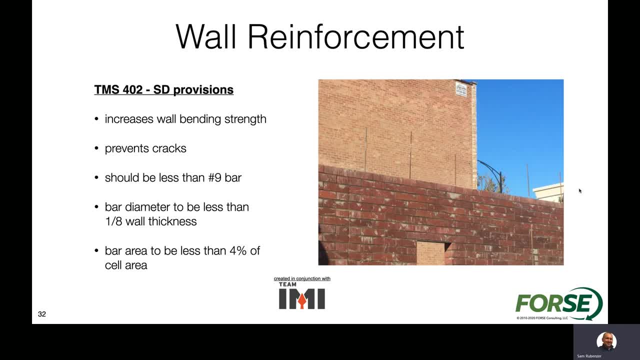 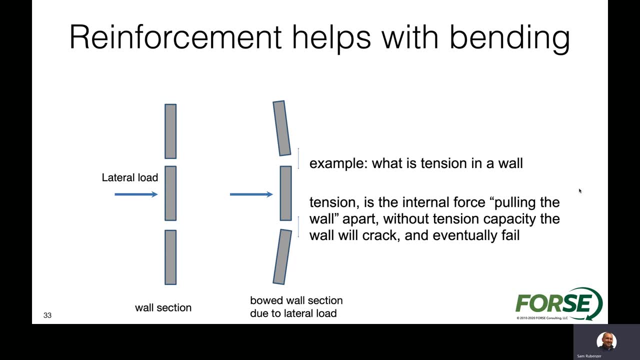 for a confined space and then the last provision of barriers to be less than four percent of the cell area. again, why are we adding reinforcement? it really has to do with any lateral load that you have on the wall. the more the lateral load, the more that we could develop tensile forces. 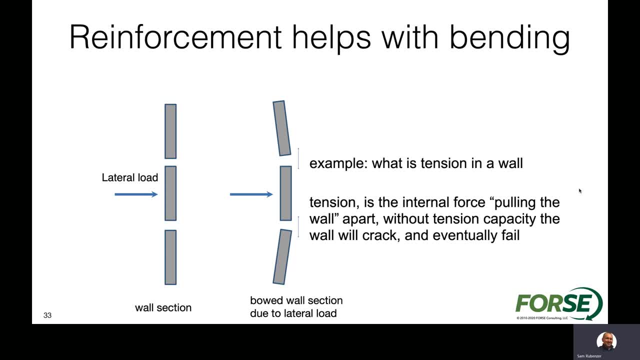 within the wall. again it's going to be the kind of that separating of the far side of the lateral load where we have a little bit of tension in the wall right. so again we have a little bit of tensile capacity. we talked about that before. if we use a certain type of 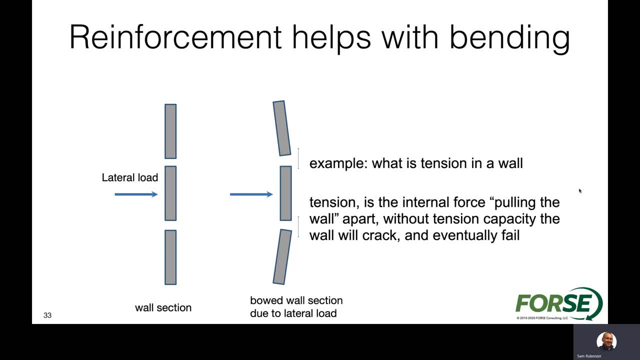 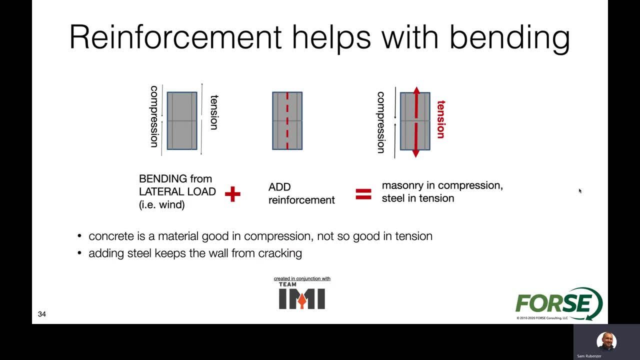 mortar. maybe we can get even a little bit more, but it's to be far less than the overall compressive capacity. so again, compressing compression and tension that you have from the bending, from the lateral loads that you have in a wall, adding some reinforcement- reinforcements that have a lot more. 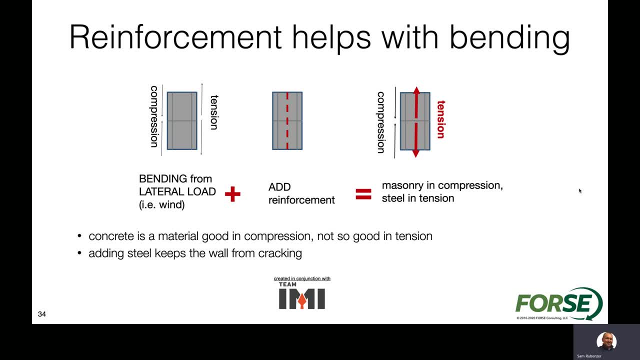 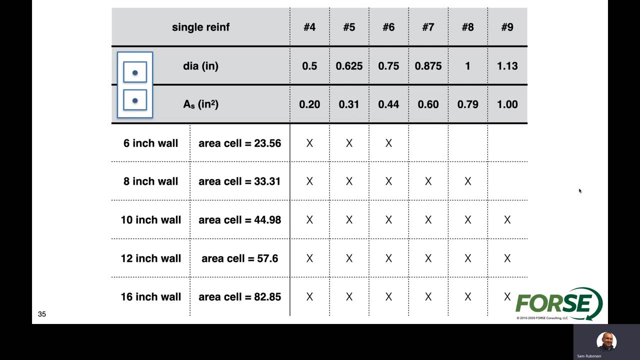 tensile properties better at tension than mainstream is going to be. so adding a little bit of reinforcement is really going to go a long way for our designs. and again, thinking about some of those provisions for reinforcement, how much reinforcement you could put in a wall really. i created this chart to really kind of point out you know fours through nines are 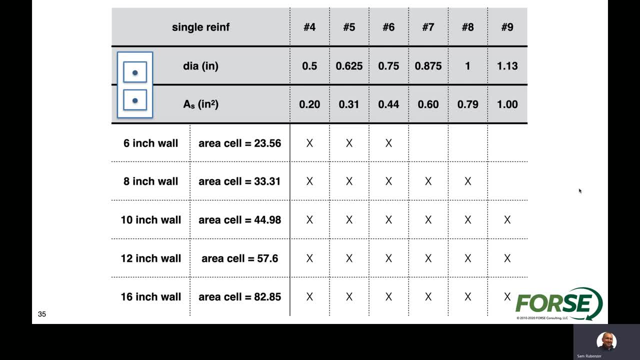 probably going to be the most common within mainstream walls and i think we can narrow that down even a little bit more, certainly on the thinner walls if we go to doubly reinforced. if you were left corner doubly reinforcing a wall, it would even limit the reinforcement that you would. 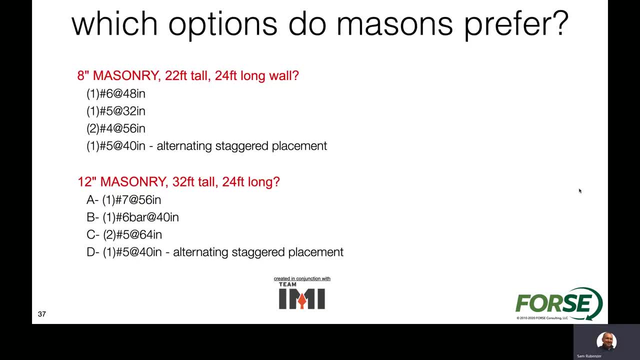 use even that much more. but i think it's always really good to think about what do masons prefer? you know we have different reinforcement schemes that we can use that achieve the similar or same moment capacity right. so for like an eight inch masonry wall, 22 feet high. 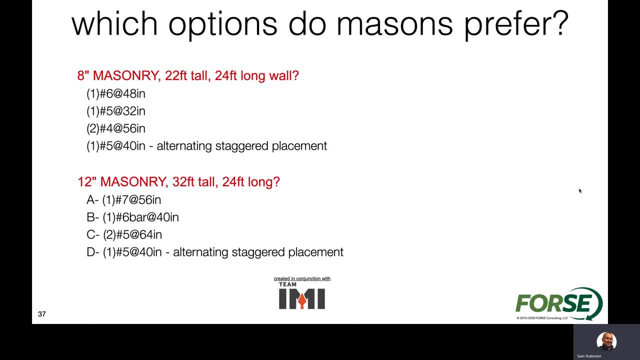 i could do a number six at 48, or i could do a smaller bar at 32, closer together, right that makes. or i could do two number four bars at 56, a little bit further than that 48. you know what do masons prefer? all of them have similar capacities and i do a similar exercise for a 12 inch wall. 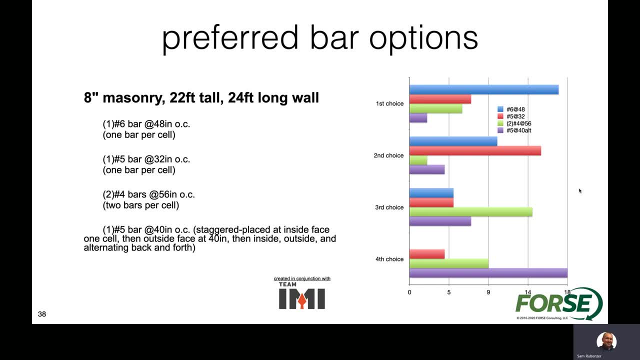 if i look at my survey results you can see masons strongly prefer the single bar. number six, you know 48 inches on center you can certainly see a few masons like the number five at 32, smaller bar, easy to work with, not a lot preferred the single bar is a little bit smaller. 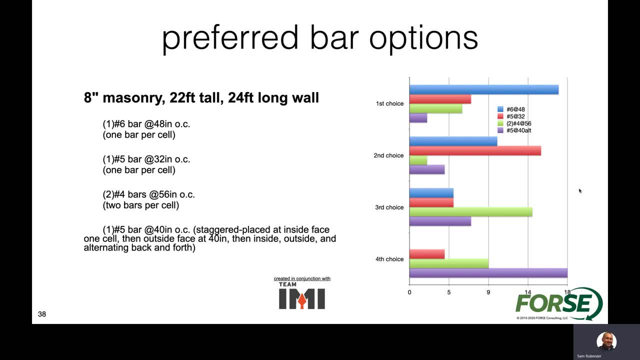 when the mason goes in between the two number four bars. again, it's just too thin of a wall. we have that confined space. putting two bars within an eight-inch wall is not going to be something that a lot of masons are going to prefer design-wise, so that makes a lot of sense. 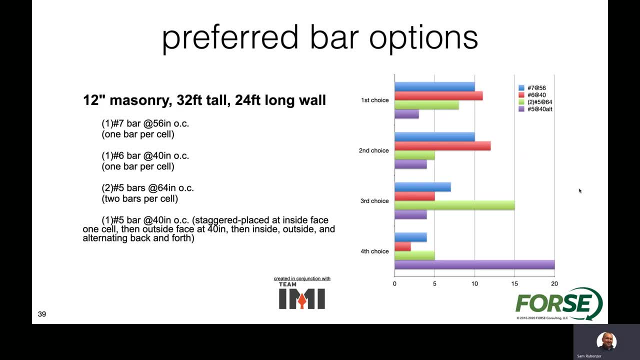 i think you can see a lot of good reasoning here, and i think we even learn a little bit more when we go to the 12 inch wall. so again we have a large bar, number seven at 56 inches. on center we have that six at forty. so a smaller bar, but closer together, more ground. 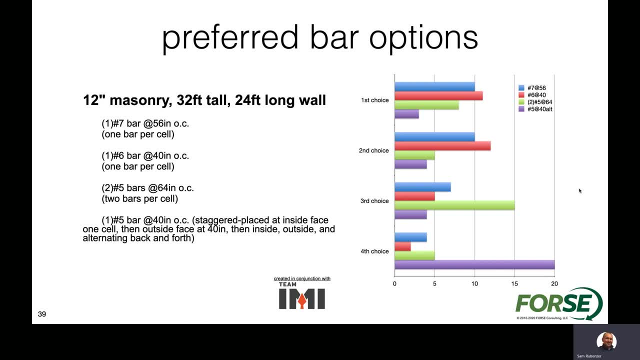 two number fives at 64.. two things that we learned here: that large bar at the furthest spacing is not as preferred as this number six at 40. that's a very interesting result. i think that you know why do masons start to shy away from that first option? it just had to do with the number seven bar number. 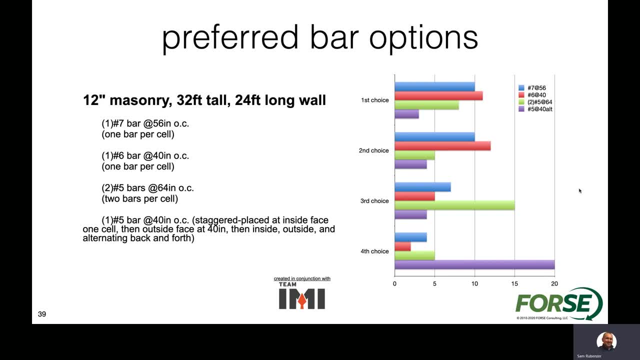 sevens are that much harder to work with than sixes. so sevens and up, there's gonna be bars that masons start to want to shy away from wanting to use smaller bars. so you can see that's a very interesting result. four, fives and sixes are going to be much more preferred. 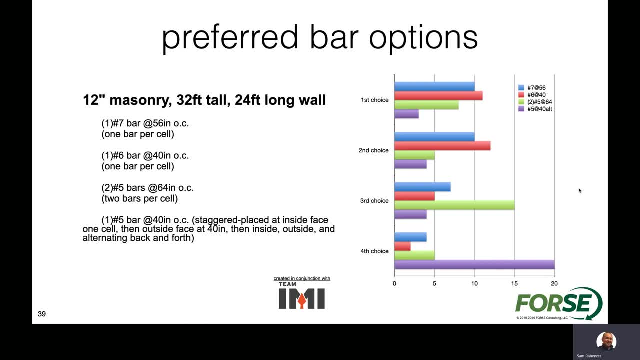 so you can go up to a number nine, but four, fives and sixes are going to be what masons would prefer. that you choose the two number five bars, that actually wasn't too far behind, right, that was something that a few masons preferred, but the two masons are going to be a lot more likely to 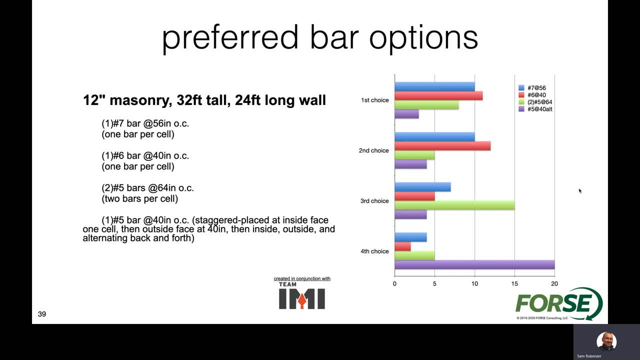 want to build a 12 inch wall with two bars. we just have that much more space within those cells. so we can see within this result, number sevens are starting to get too big. uh, two bars and a thicker wall do make a lot of sense. two masons, so pretty good information there. 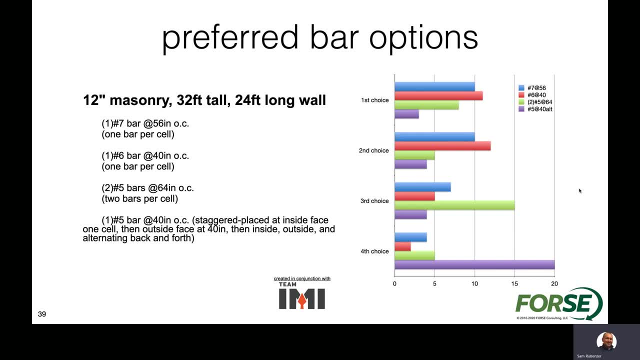 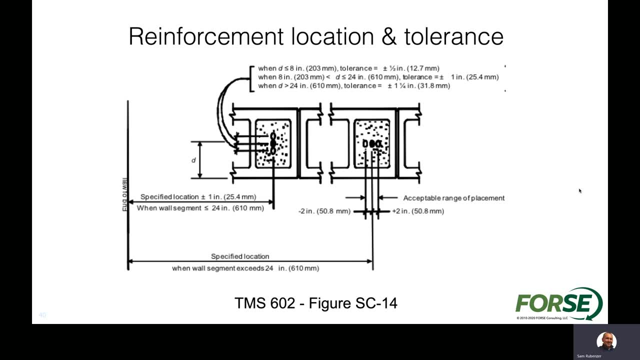 i think that we can take back, as we develop some of our designs, other things to recognize and really this slide. i put this in there really for making sure that as you go to the field and you look at where reinforcements placed within a wall, we may specify the reinforcement to be. 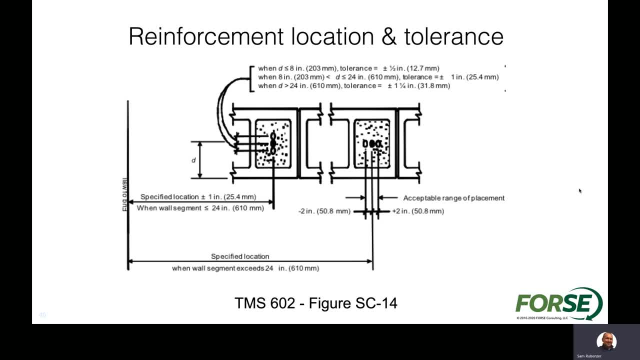 centered in a wall. but this is a really good guide. again, within tms 602 that shows you, with an eight inch or thinner wall, a bar in the center can be plus or minus a half inch from that center line. if the wall is greater than eight- say a 12 or 16 inch wall- then we actually have plus or minus. 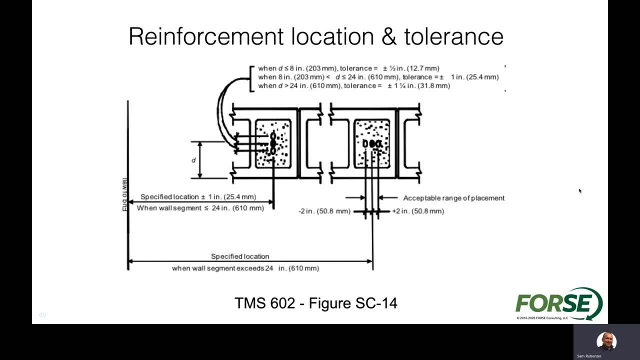 one inch. um, so the code's going to be building in all of that uh tolerance when it develops those capacity equations and so on and so forth. so we really need to recognize that this is a construction tolerance. that's just fine. the bars can be a little bit off center within that. 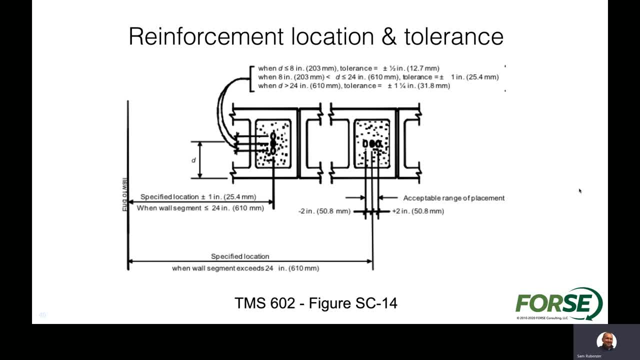 tolerance as they build the wall, which gives masons again a little bit more flexibility and engineers can keep their minds at ease as we go out and we look in the field and we see some of these bars placed within mason walls. just understand the tolerances that are built into the code equations. 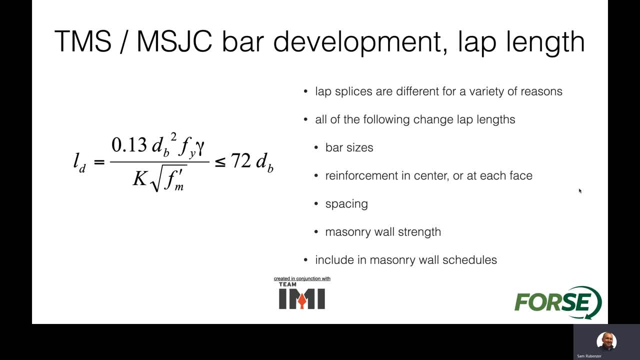 next thing with reinforcement: lap lengths. lap lengths are something that can be a little bit confused. uh, for masonry design, there's a pretty straightforward- well, pretty straightforward- equation here. um, that's developed within tms. we can certainly develop different lap lengths for different situations: for mastering walls, the bar size, reinforcement in the center. 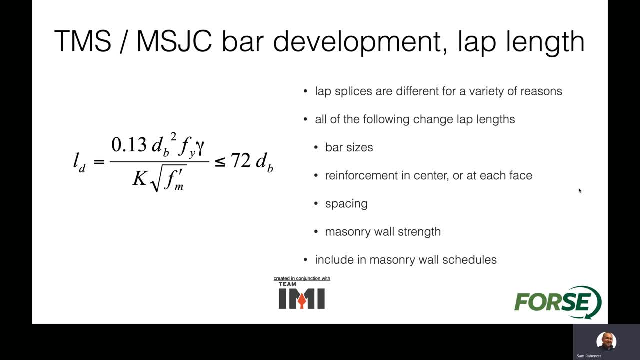 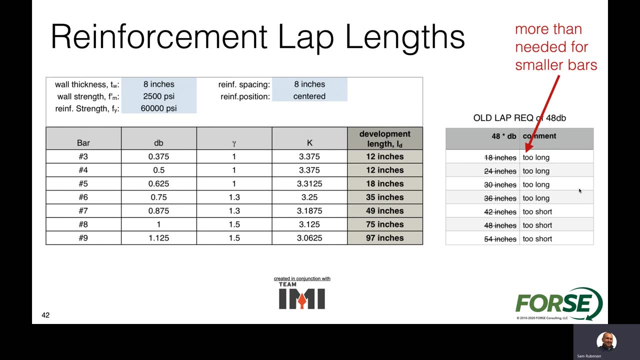 at each face spacing or overall. all of those different variables can actually change what the actual lap lengths could be for the masonry walls. if i take that formula and i put it into a spreadsheet, you can see that it's pretty easy to see what the actual lap length development. 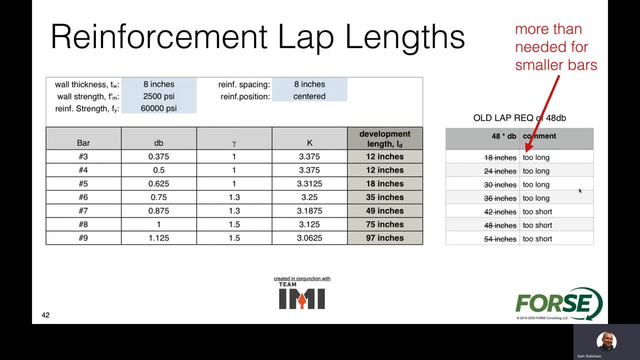 length is going to be for different size bars for different situations, and the one thing that i also want to do is compare it to what i would call the old lap length requirement, the 48 times the diameter bar. if you see my comments there, you can see for the first four, for number threes, through. 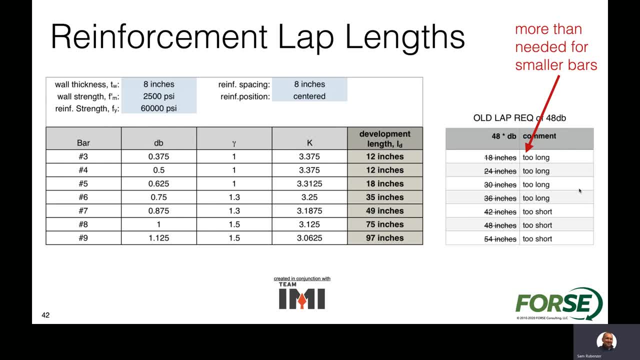 number sixes. uh, the number six is the value of the bar. so what you're going to do is you're going to. the development length is just too long. It doesn't need to be that long. so that's just wasted reinforcement you could think of on your projects. Number six is it gets pretty close. 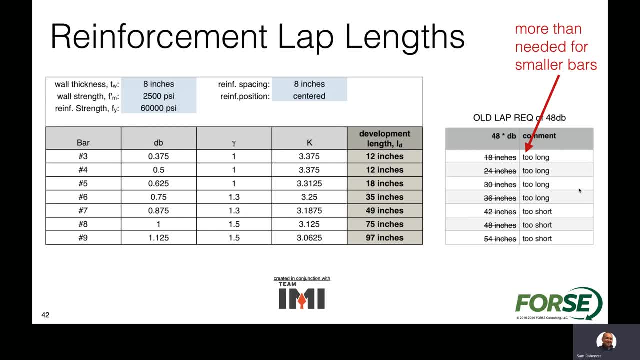 but the really interesting thing, I think as well, is sevens, eights and nines. the actual 48 times diameter bar is actually too short, So unconservative is definitely not something that we want to get into. The other thing that we want to remember here is: this is all dependent on. 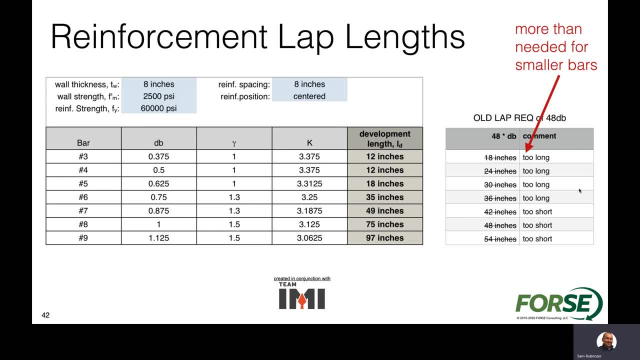 a few of those different variables: f, prime, m, spacing of reinforcement, whether the reinforcement's at the center and at each face. Really, I think when we develop lap lengths it could be, there could be a situation where we have the same bar. there's two different lap. 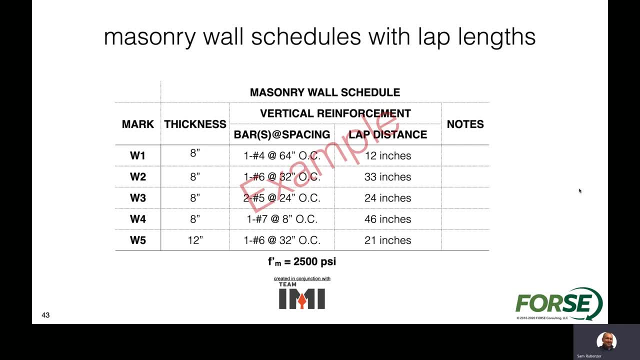 length center projects right. So this example: if I look at W2 and W5, they both use number six bar. With W2, I actually have a 33-inch lap length. Well, W5, I have a 21-inch lap length. 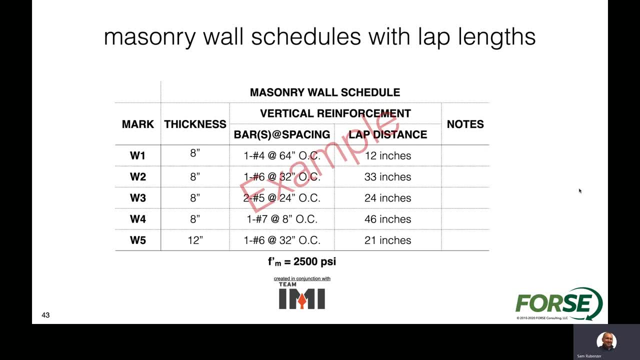 for that number six bar. So I think that's really interesting to look at and think about. you know, maybe my W5 is the most prominent reinforcement for this project. I have most of my walls 300 feet by, 300 feet by, you know, 34 feet high. They're going to be a 12-inch wall. 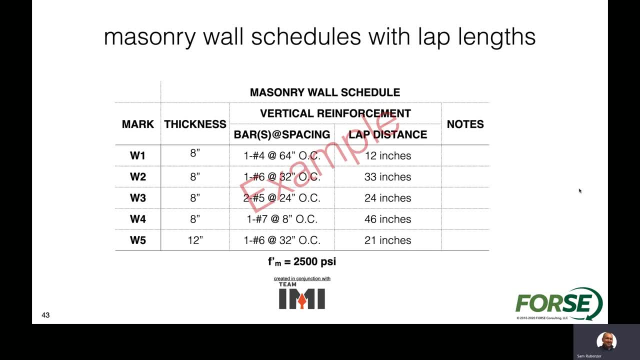 with that reinforcement. I don't want to have that lap at 33 inches for all of those elements if that eight-inch wall is just used for a little screen wall on the project, right? So maybe a schedule and actual lap lengths within that schedule? This is really clear for contractors. 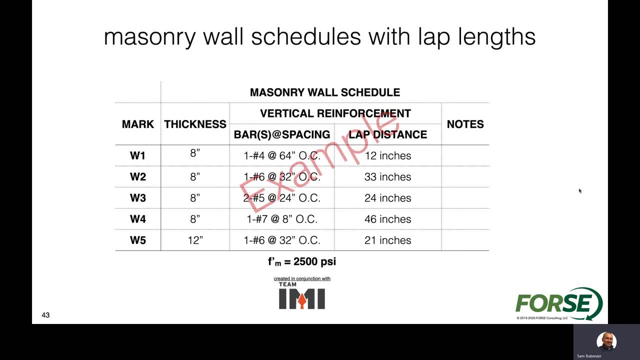 They can certainly look at this chart pretty quickly and see what laps they need to use in different areas of the project. It also gives you know what the reinforcement needs to be. I think that's just a really good and clear way to do it, So something that we suggest. 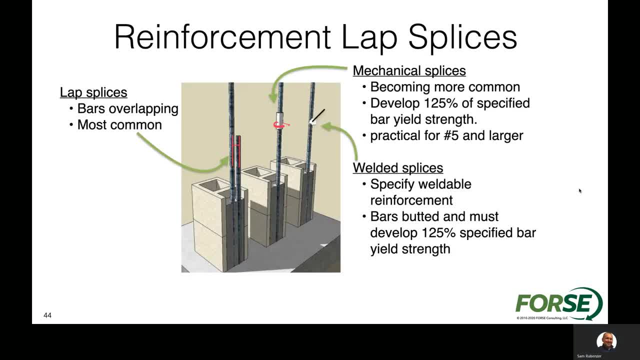 engineers consider. So we talked certainly about lap lengths. These are different ways that we can splice reinforcement. Absolutely Well, let's splice it, Let's splice it, Let's splice it. Splices are certainly available. That's not going to be too common, either in concrete or 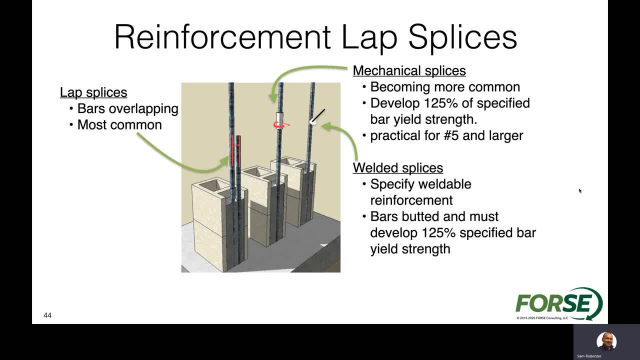 masonry construction, but that's certainly something that's available. Mechanical splices are something that we see used quite a bit within concrete design, and I'd like to see them used a little bit more with masonry design, Certainly as we get into some of the larger bar sizes. 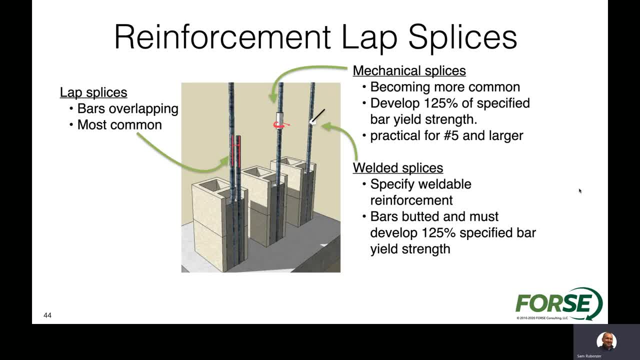 using those mechanical splices, especially the threaded couplers, can be very nice within these confined areas in masonry. There's certain contractors actually that prefer to use threaded couplers only to develop their bars Makes it a lot easier for them construction-wise. So I would say as engineers we don't have to specify something else, but just. 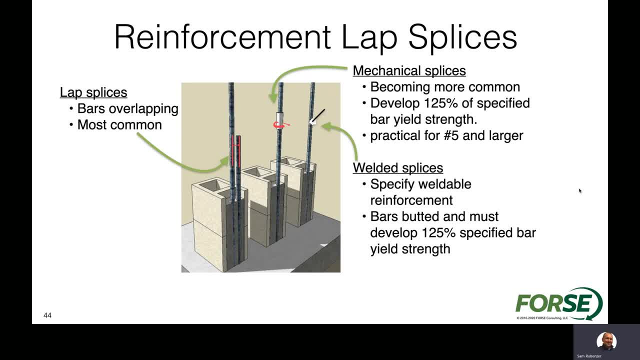 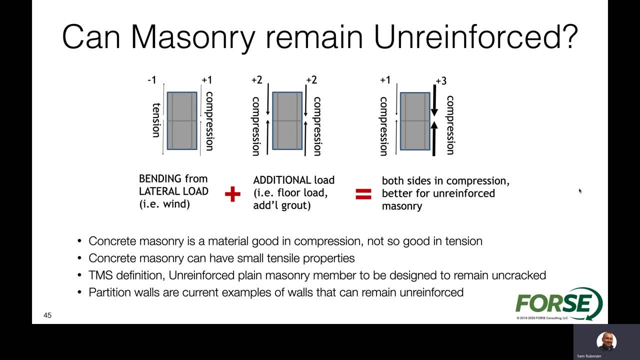 be open to and recognize that different contractors might be requesting this. So all that talk about masonry: can masonry remain unreinforced? the answer is it actually. can You know? we can go all the way back to that chart on mortars. You can see that there is some tensile capacity that we have. But the other thing, 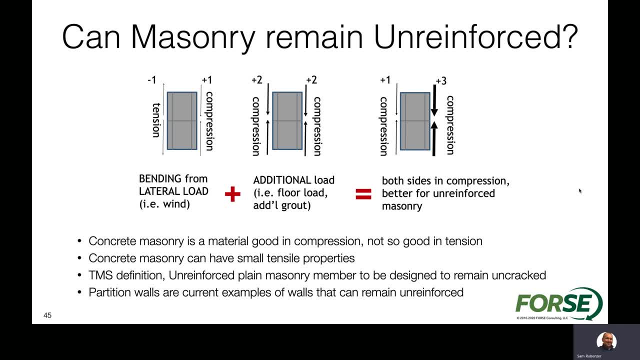 about masonry is if you just add enough load to it. you know, if I have that bending that I have in my wall, it creates certain tension and compression forces. If I just have enough vertical load, say a floor load, that actually balances out that tensile force and keeps both. 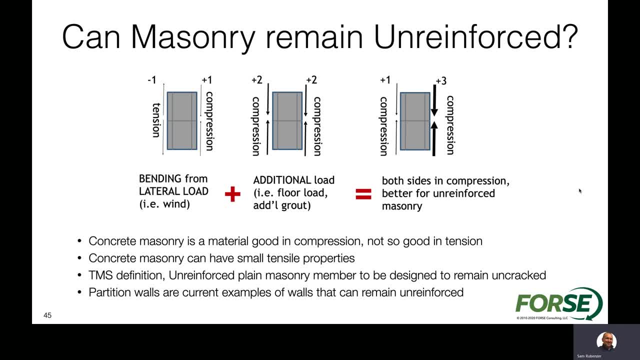 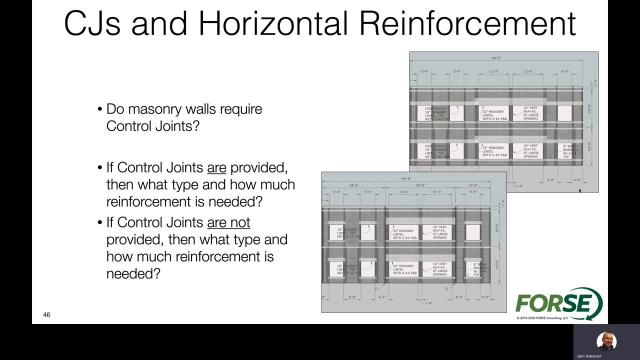 sides of the masonry wall. in compression we still have plenty of opportunities for unreinforced masonry, But I think likely some reinforcement is going to be used for most masonry these days. Next we're going to switch over to control joints and horizontal reinforcement Again. 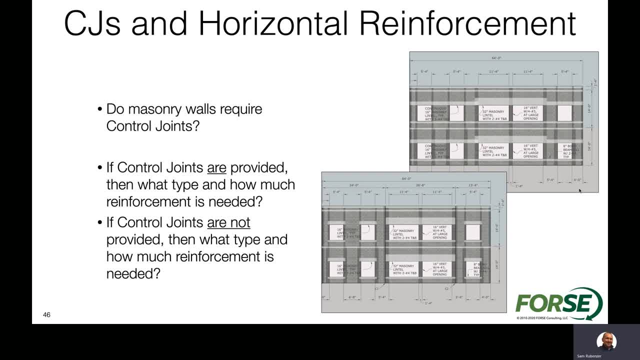 mostly control joints are going to be used for walls that have light reinforcement. Control joints can be provided Certain levels of minimal reinforcement can be used. But there's certain situations in designs, in all different seismic design categories. control joints maybe just aren't necessary because we have so much horizontal reinforcement already. 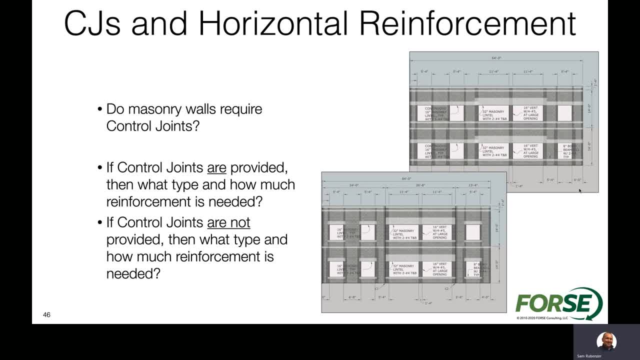 within the wall that we don't need to provide control joints. We have sufficient reinforcement to prevent any shrinkage or temperature cracks from developing within the wall, And so it's just kind of a modification for how we look at the masonry walls and how we can simplify them. I would say by taking some control joints out for different projects. So something that's really important, I think, for one is banking. So, for example, if you actually need a control joint villain wraped, you're either going to have to do somebody else or another, whereas a masonry is really anől that's going to be required to create control joint. 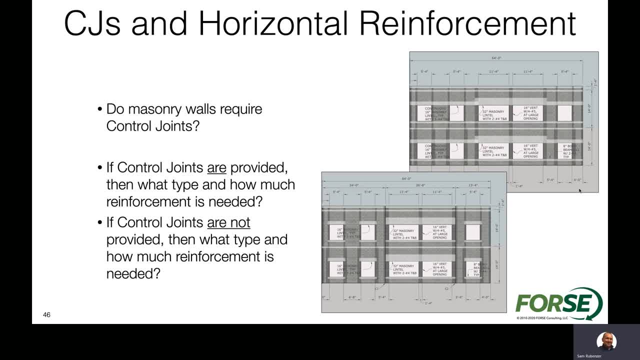 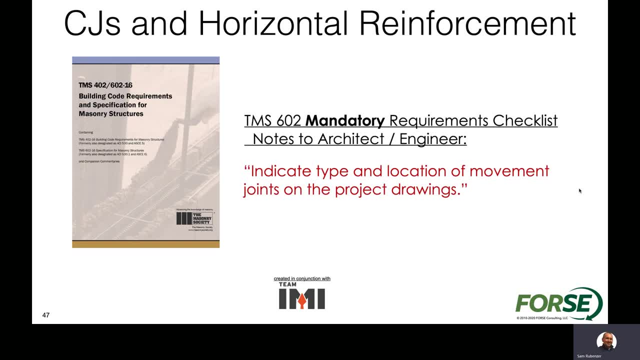 say, by taking some control joints out for different projects. So something that's really important, I think, and we'll talk about this maybe more in a different presentation. but you know, making sure that you locate control joints are certainly the responsibility of designer. 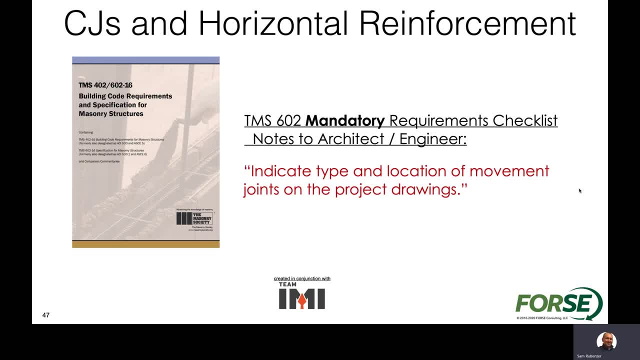 The TMS 602 mandatory requirements actually indicates that it's the responsibility of the architect or engineer to indicate the type and location of movement joints on project drawings. So that definitely includes control joints and certainly as an engineer that's trying to have a very good understanding for structural masonry design elements, I think it's very 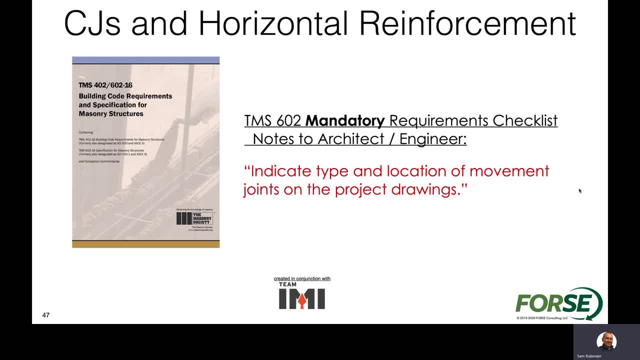 important to have a good understanding for exactly where the control joints are, and I definitely would want to then specify them and not try to guess where a mason's going to provide them based, because if you provide vague information for where the control joints go, then that's really what you're left to: trying to guess where they might put them. 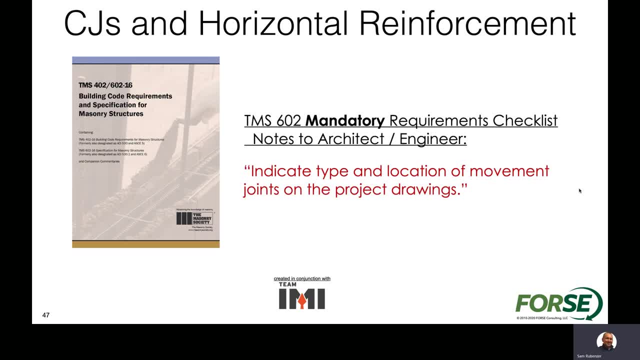 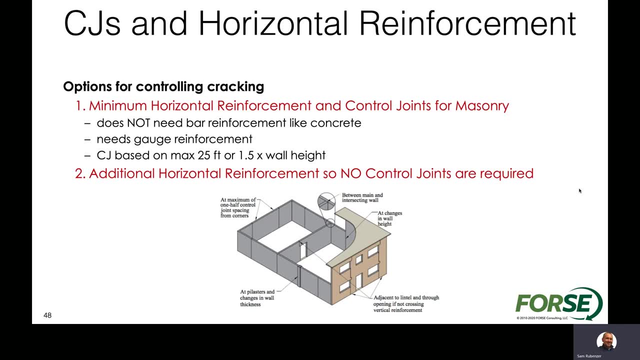 So I think specifying their exact location is definitely the situation that we want to be in. For this we're going to rely on. this is an NCMA Tech Guide 10-2D that has this diagram and these recommendations for minimal reinforcement and control joint for masonry. but there's 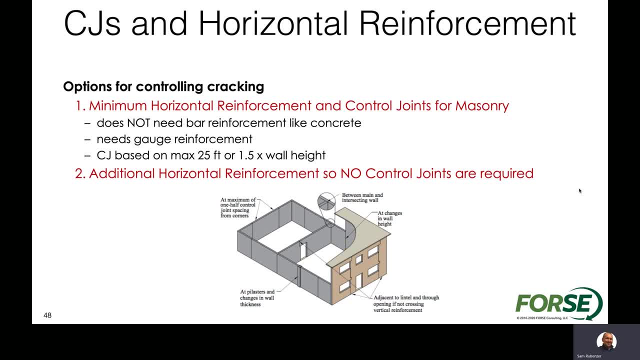 a different NCMA Tech Guide. NCMA Tech Guide 10-2D has a different NCMA Tech Guide 10-2D that has a different NCMA Tech Guide 10-3 that looks at the amount of horizontal reinforcement that you need. 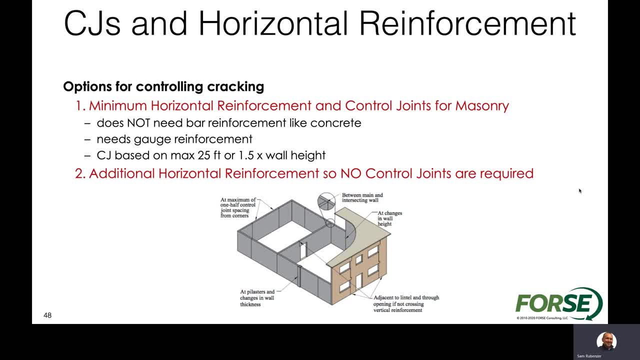 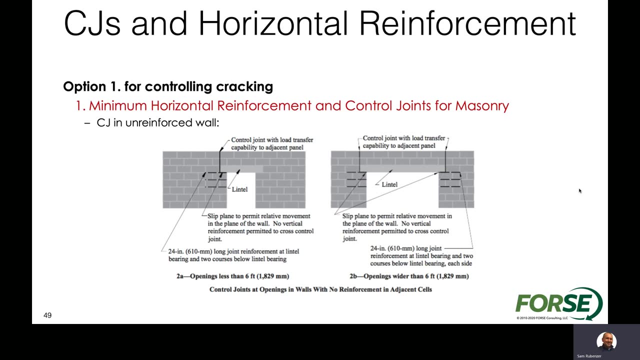 so no control joints are required, and so you really have those two different options for controlling cracking within masonry walls. If we focus on the first one, you know the minimal reinforcement, the first thing that maybe we want to look at is: well, what do we do at windows if we have that minimal reinforcement? 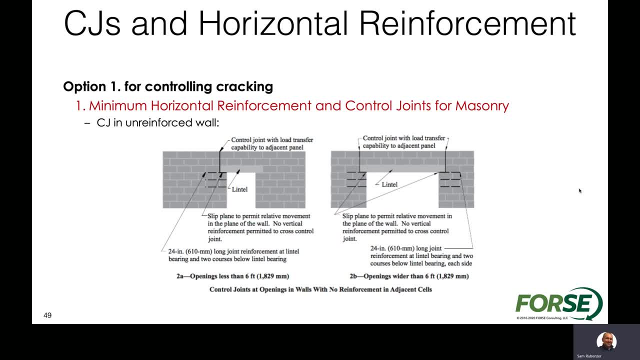 and control joints and we have an unreinforced masonry wall. We've talked about why most walls have some level of reinforcement. There's a few walls that can still be unreinforced. In those few walls that are unreinforced, this is where we're going to put the control joints. 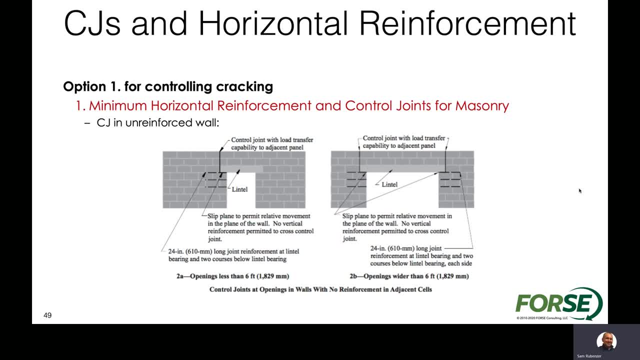 at the opening edges or develop from the corners of the openings. You're going to have some stress concentrations there. You would have a crack that would want to develop from those corners, and so if it's an unreinforced wall, then we can look at putting those control joints at the opening. 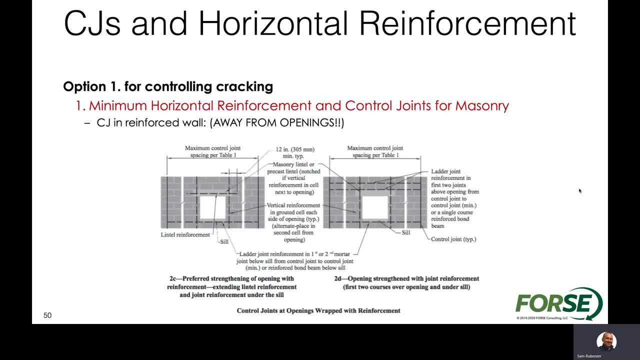 edge. The much more common structural masonry wall is going to have some level of reinforcement. Again, reinforcement around openings is very, very common. You have jam reinforcement, You have lintel reinforcement. In that situation, again based on this guide, we're going to put control joints away from 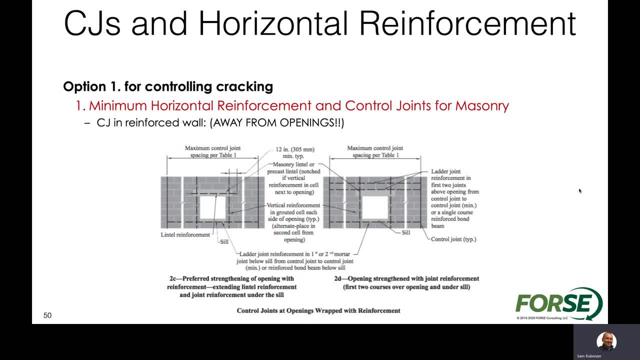 the edge of the openings I would say away from the openings could be eight feet. It could be four feet Probably doesn't want to be much less than two feet, maybe 16 inches, Certain situations, But the further you can get the control joints away from the opening when it's a reinforced 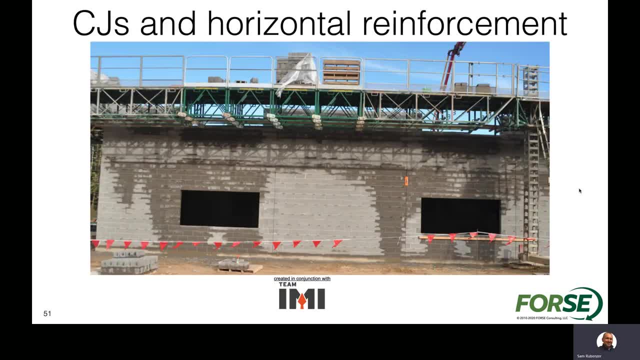 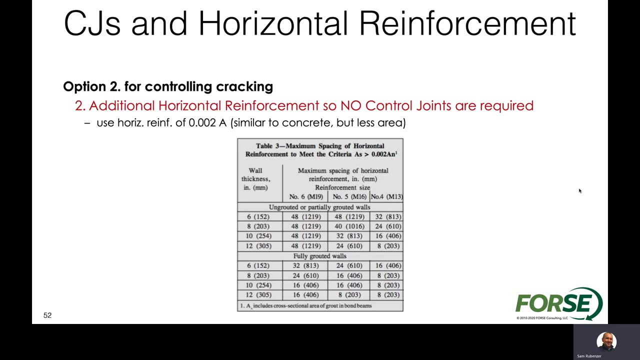 masonry wall, the better. Just a really quick example of that is. here's a wall with the opening. You can see control joints on each side of the opening, two feet away from the edge of that opening. So again, we're talking about placing control joints when we don't want to have control. 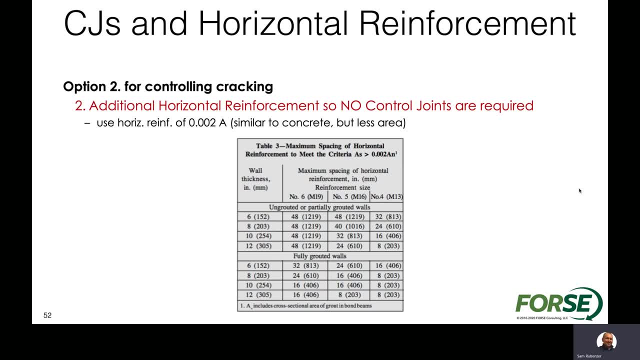 joints required on a project Probably still put some of them in for certain situations, maybe changing wall height or change in support conditions would still require control joints. But so that we don't have to put them at a regular spacing within a project, we simply 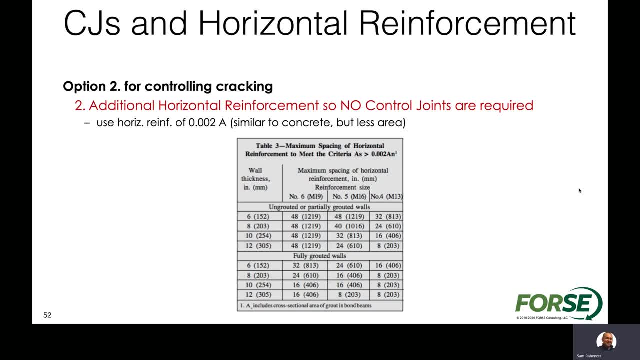 have to meet a criteria for reinforcement of 0.2% of the overall area of concrete. So it's going to be a similar provision to what you'd have say in the concrete code, But with masonry we just have less concrete. 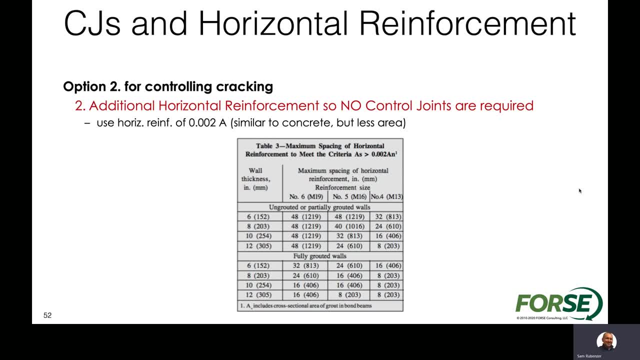 We just have face shells. when we have ungrounded or partially ground walls, that face shells are going to be the only control joints. So we'd have a lot less area of concrete that we can consider. So we'd have a lot less horizontal reinforcement that would be required. 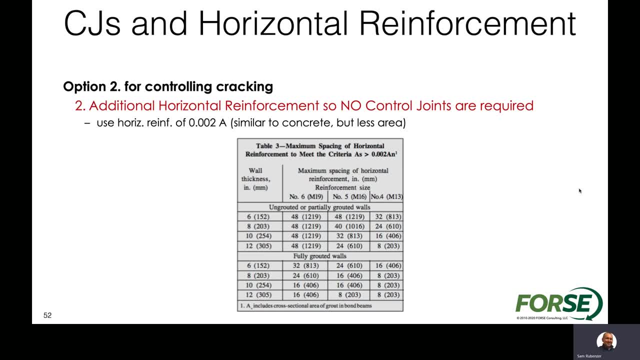 If we get into a fully grouted wall then we would have to add a similar level of reinforcement that you would have in a regular concrete wall. Fully grouted masonry walls are going to have a lot more horizontal reinforcement required And you can see that in the chart below. 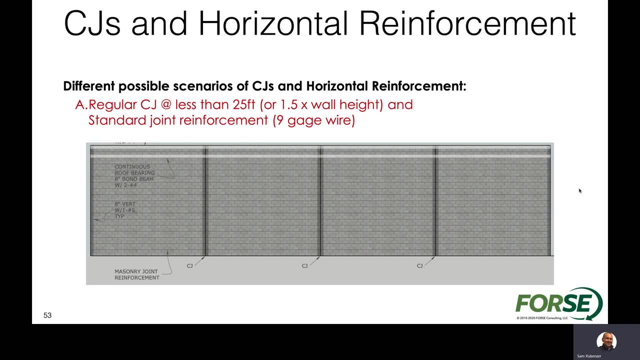 So again, if we look at and consider different schemes here, For a typical wall, if we have control joints at regular spacing, then we would have possibly standard joint reinforcement that could be provided. That could be one method for this horizontal reinforcement scheme for this masonry wall. 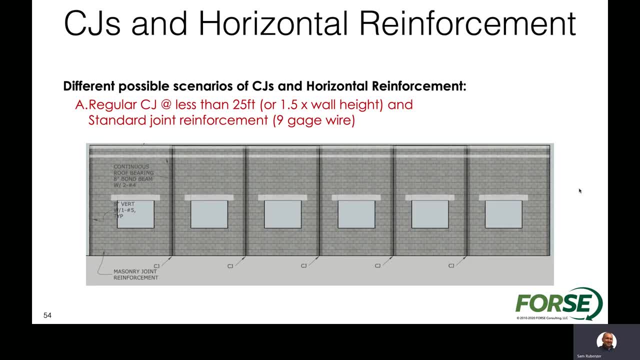 If I had openings to consider. certainly that might change where my control joints go. I might have to add some control joints to make sure that my control joints fall between these openings. It doesn't get too close to the edge. But again, mainly it's going to be control joints plus horizontal joint reinforcement. 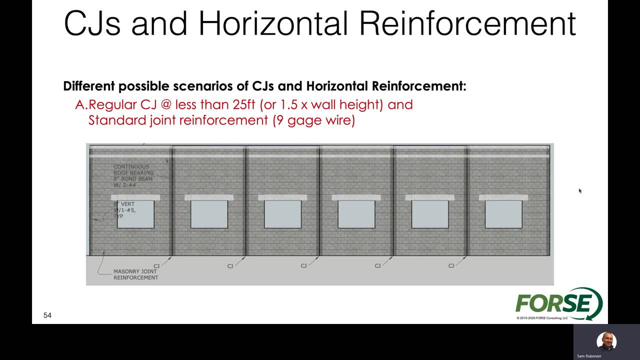 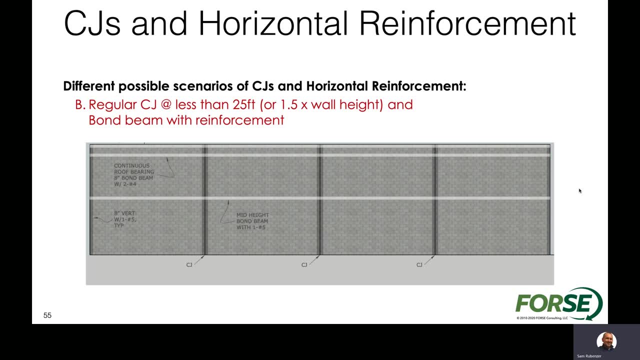 And this is another option for reinforcing this masonry wall Instead of joint reinforcement- another option that we have if we want to use regular control joints- what we can do is we can add a mid-height bond beam, provisions for the bond beam being. 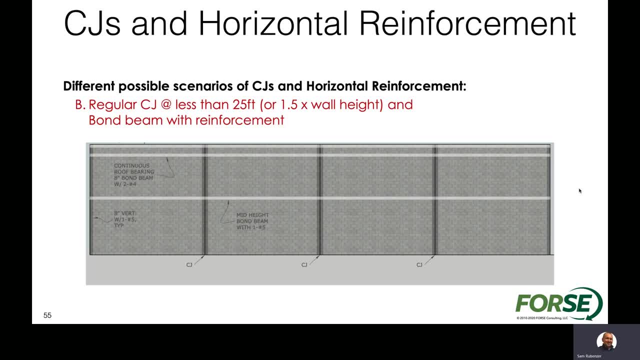 within the wall no more than 12 feet On center and then have enough reinforcement based on the overall of masonry that we're needing to reinforce. So certainly this is another option. We have a lot less reinforcement in terms of quantity. 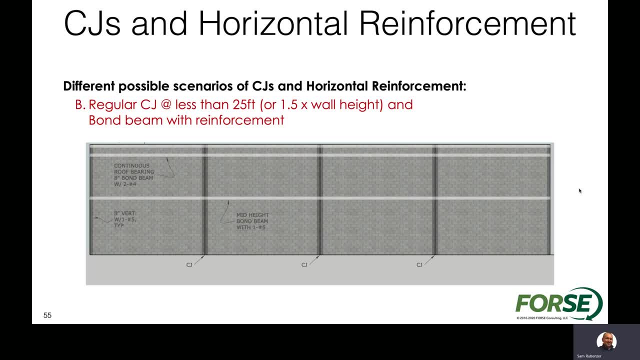 Instead of having joint reinforcement, every other course- providing a mid-height bond beam and say a bond beam at the top or maybe a couple at the top because you have some bearing conditions- is just another option for reinforcement. So we can do that. 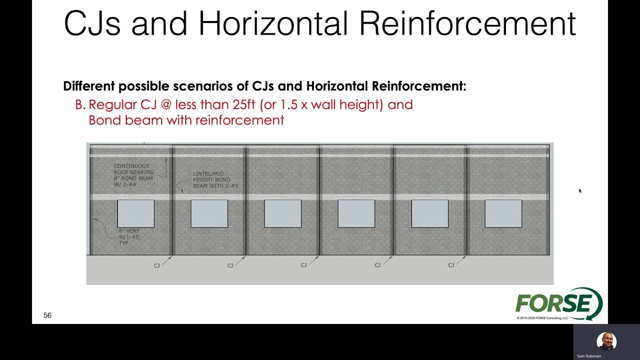 And then we can add a masonry lintel for this wall with control joints, And this is just a look at what that could look like if we have again those openings. Maybe in this situation, instead of having that mid-height bond beam, because we already 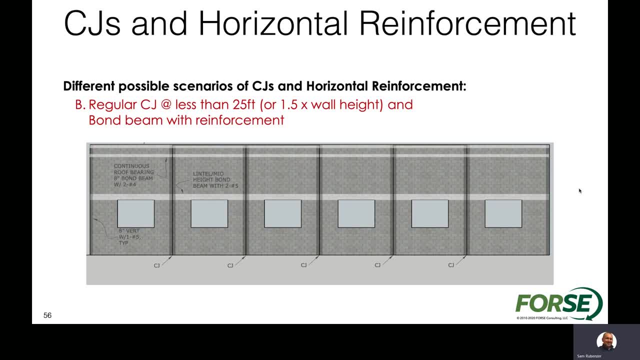 have a masonry lintel that we would use for spanning that opening. maybe we just make that continuous. So really it's using similar materials that we would have there already for the opening And then just take that reinforcement continuous to the control joints. 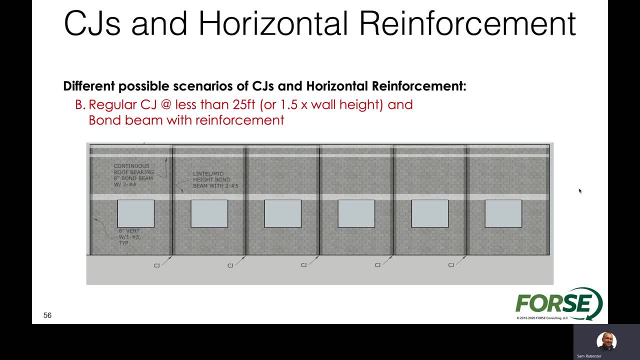 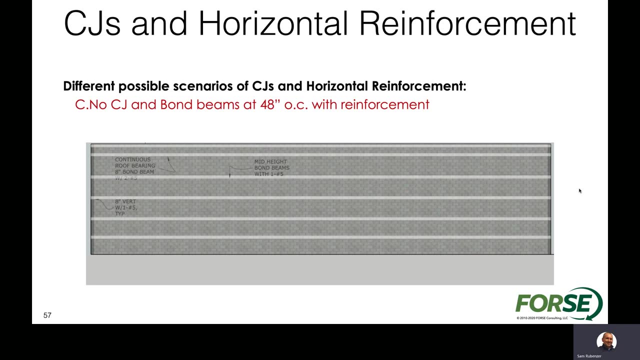 So that can be done, So that can maybe simplify this design, instead of having a lintel separately, then a bond beam and the bond beams at the top. So just another option for control joints and minimal reinforcement for a wall. So our next options here is, you know what, if we want to look at this wall and not have 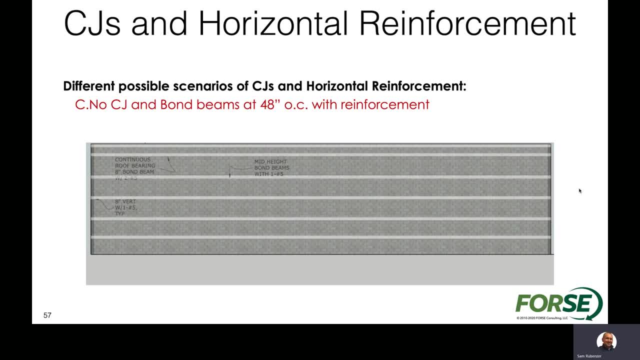 any control joints. One of the options would be to add enough horizontal reinforcement that's continuous within the wall To prevent any These shrinkage in temperature cracks from occurring. So then we really don't have any requirements for where control joints would need to be. 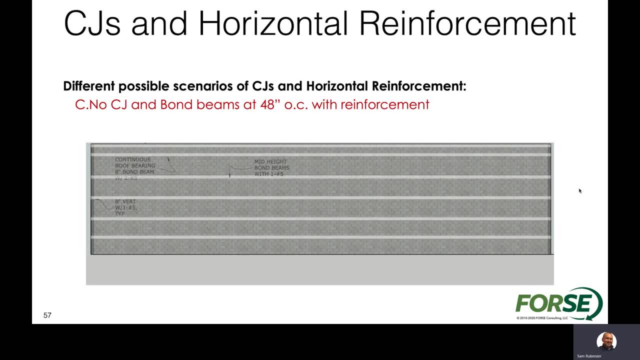 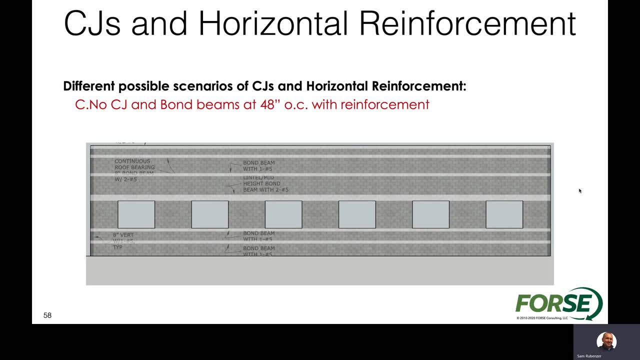 So a long wall like this with similar bearing conditions could really not have any control joints. If we again look at that same wall with those openings, this again might be the simplest way to look at reinforcing this wall. You know we have the lintel that was already there. 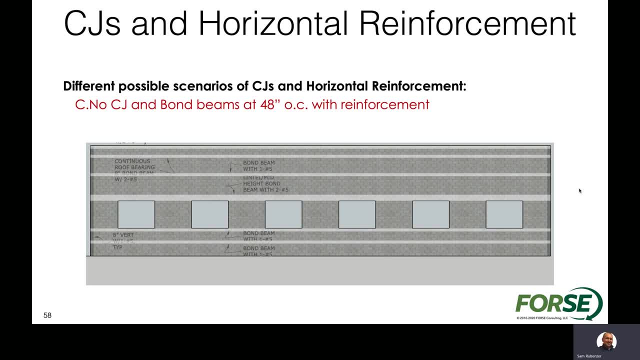 We have a top of wall bond beams and maybe a roof bearing condition. Maybe it's just a couple of the bond beams that we add to this wall That can help us eliminate all the joint reinforcement and eliminate all the control joints. That might be a lot simpler, much more cost effective way to look at this wall. 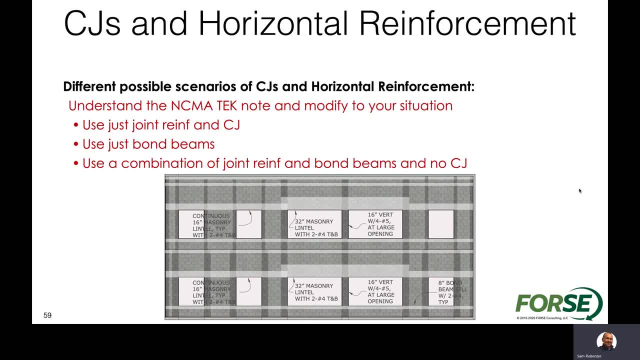 So again, just kind of recapping here, just understanding what the actual requirements are. We don't have to have control joints If we want to use control joints. we can use a less amount of horizontal reinforcement If we have a design that's already has plenty of. 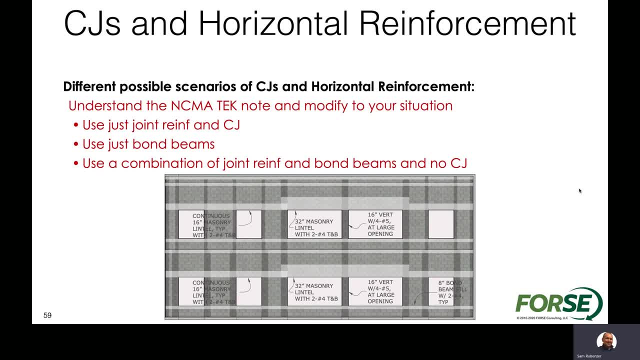 Horizontal reinforcement because we have openings, we have lintels that maybe just need to be then made continuous. Then what we can do is we can relook at where control joints would want to be, maybe eliminating some or all of the control joints on a particular wall panel and just use bond beams. 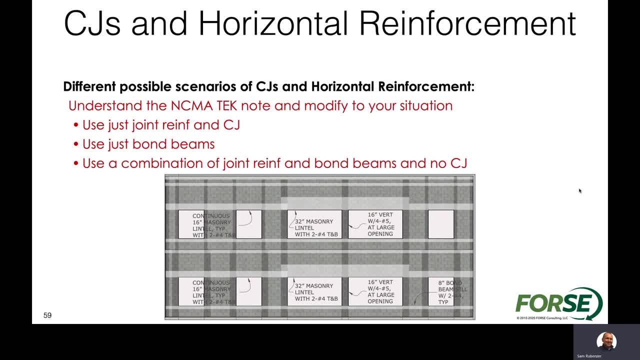 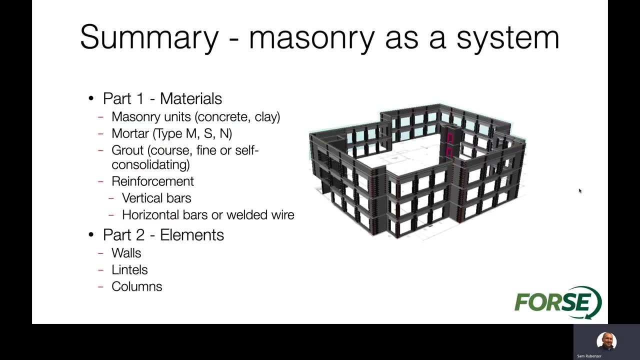 So a combination of joint reinforcement and bond beams can also be used to eliminate some of those control joint requirements. So just recognize the different options that you have, which can lead to a much more productive and possibly more cost effective design. So that's going to wrap up the first part of this talk on the materials. 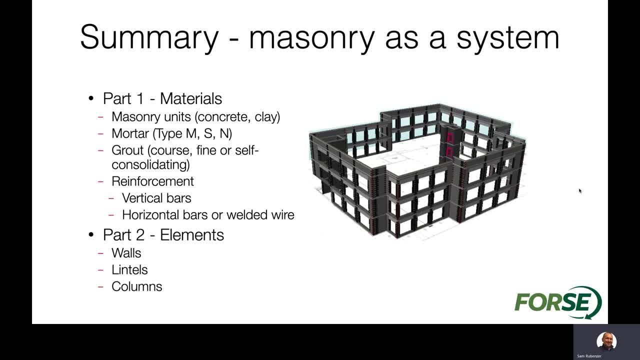 You can see that we talked about masonry units. different masonry units can be used and specified- Really want to make sure that we understand what the actual strength is of the unit, Using the right mortar type. again, predominantly we want to use a type S mortar for our design. 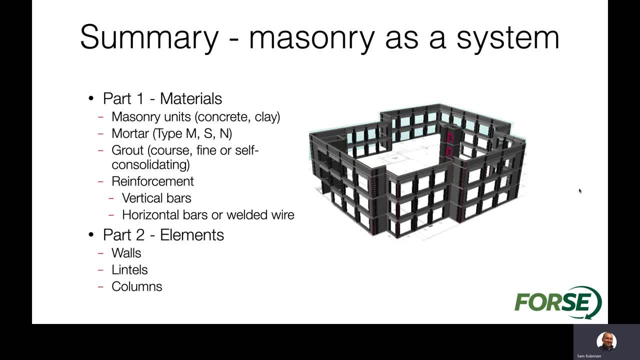 Grout. We have different types of grout as well: coarse, fine or self-consolidating. I'd say, as engineers, what we want to do is we just want to get familiar with the different options for grouting and grout pours and lifts, reinforcement, and what types of grout we maybe.